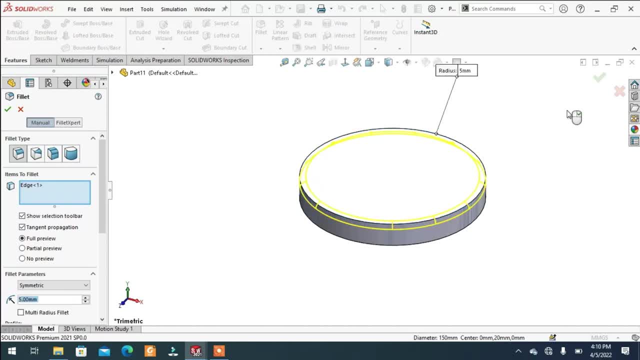 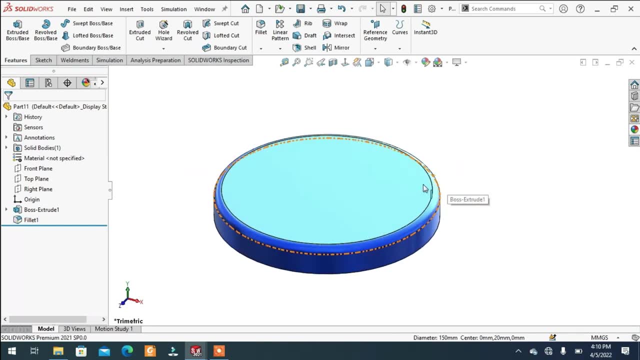 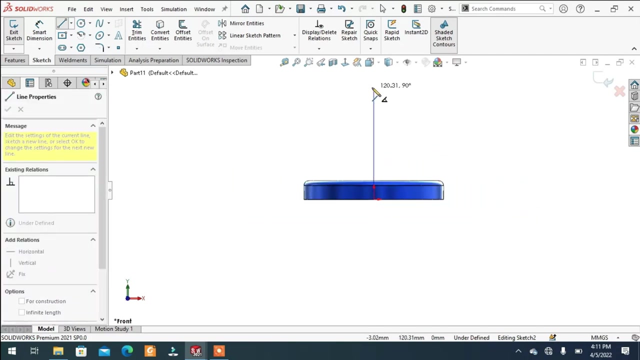 click on the edge and choose fillet and set it 5mm and you can have any type of colors and choose front plane and sketch, choose line and draw a central line. to do that, right click and construction geometry and again type s and draw a circle at the top and draw an arc. 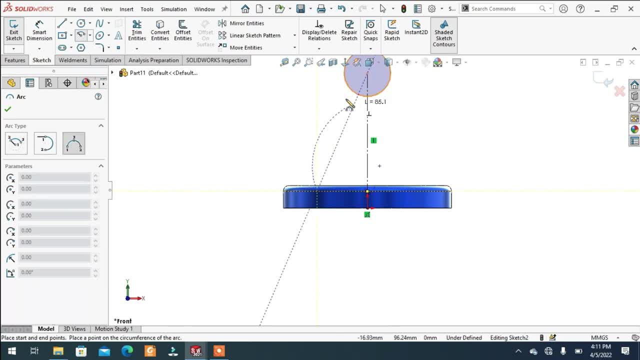 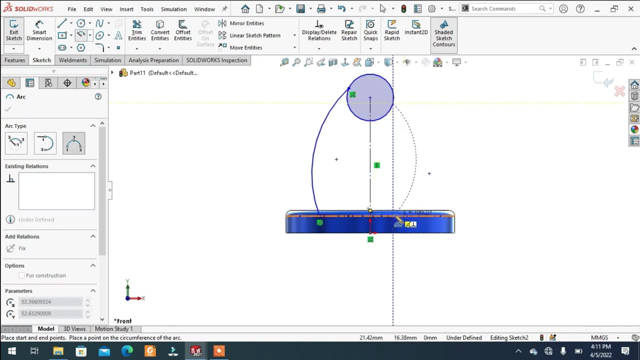 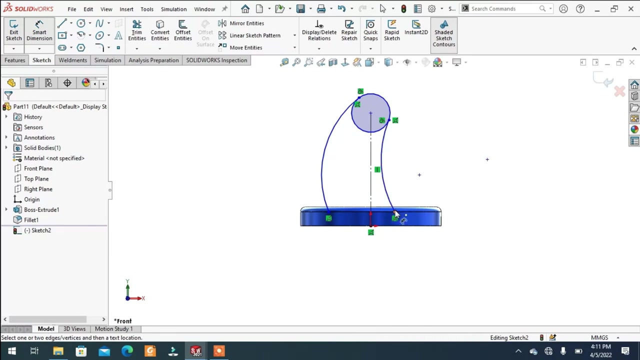 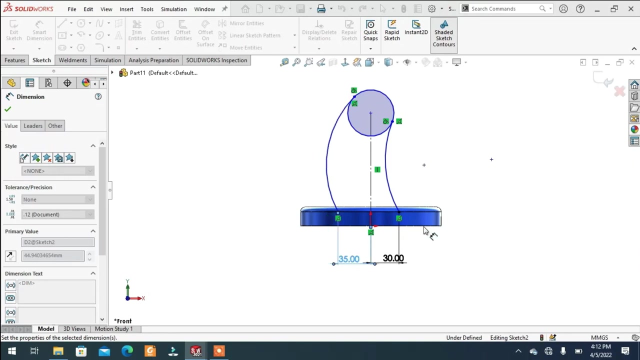 for the body of the first part and make sure these two are the circle and arc- are tangent, to get a better surface. finish at the end and give it a dimension and define the height of the first revolved joint to 100 millimeter and this circle to 30 millimeter. 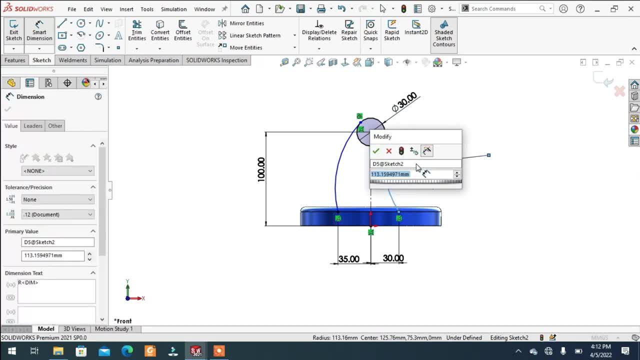 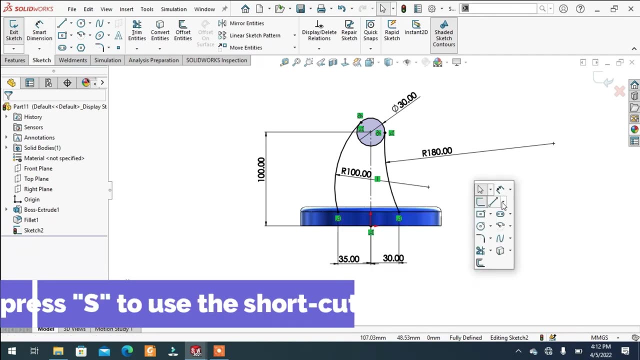 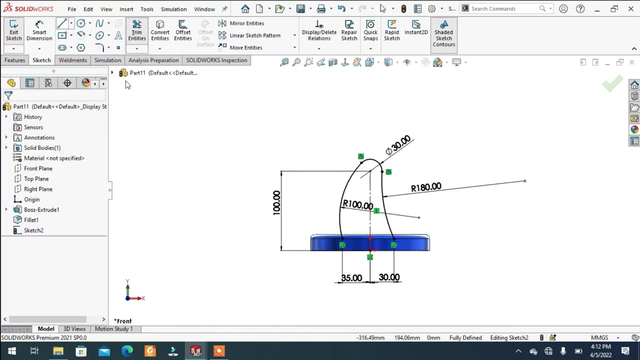 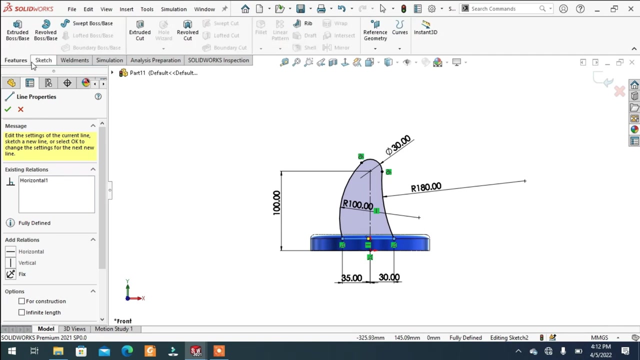 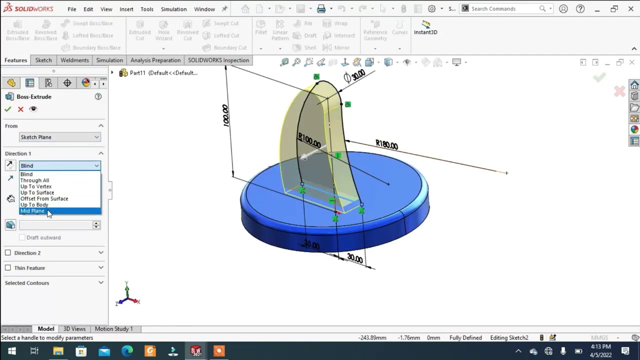 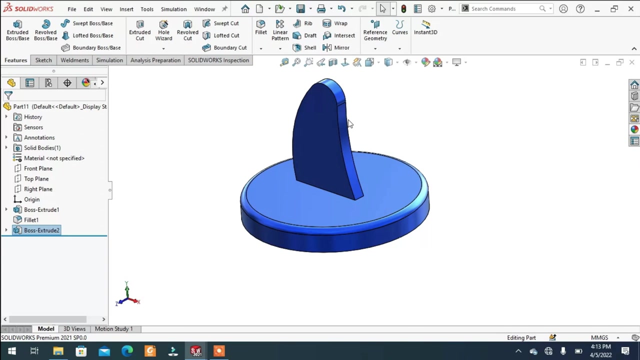 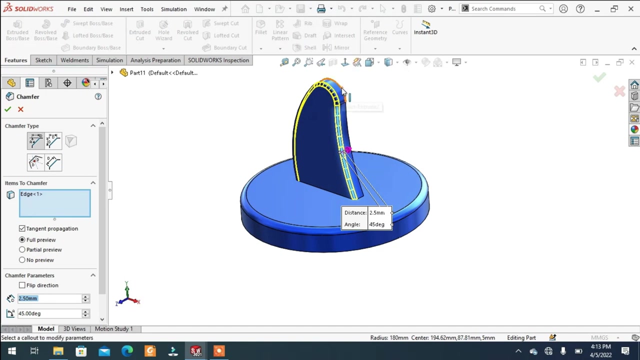 and it is not still fully defined. so define the arc, the first arc radius and the second one and the second one. then using power train command we can remove unwanted lines and close this sketch, then extrude it on mid plane and for better surface finish and strangles we can add a chamfer on the edge. 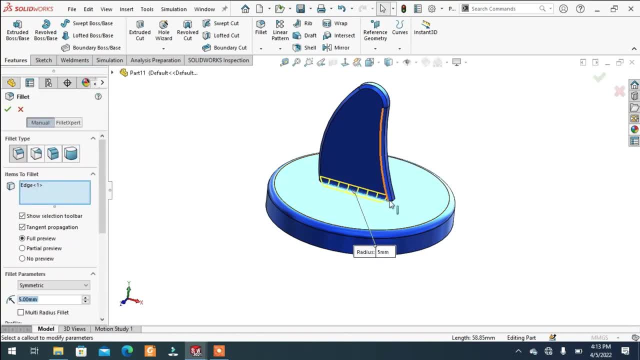 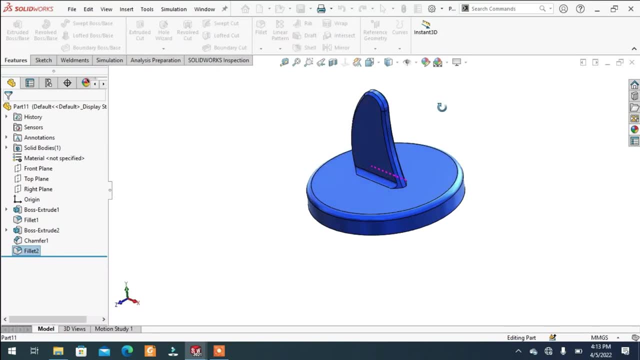 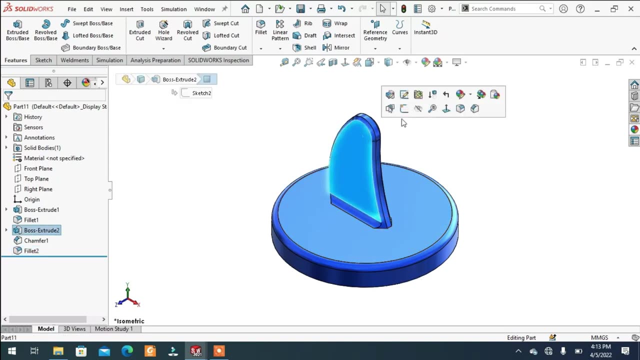 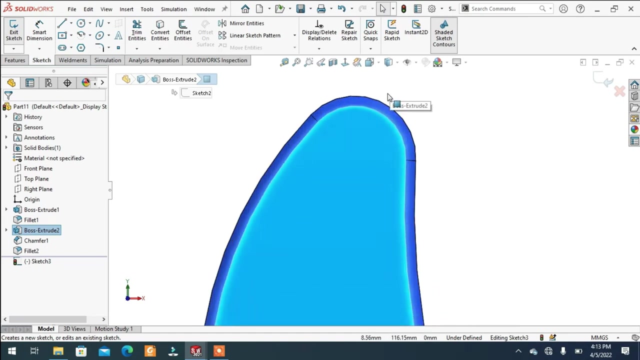 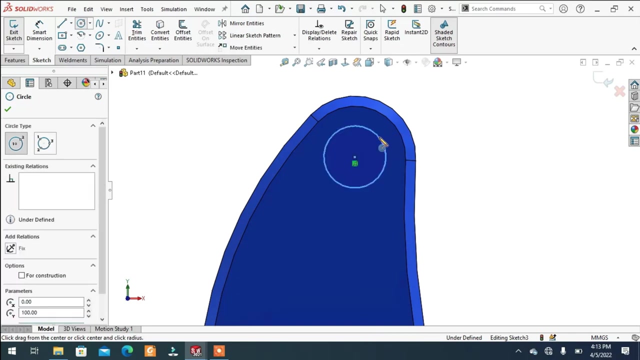 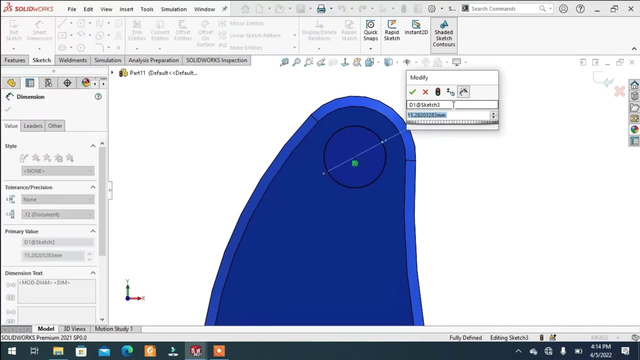 you can also use fillets. you can also use fillets. you can also use fillets. select this face and sketch. we can draw a circle, set the diameter of this circle as this circle to 20 millimeter and extrude it around and extrude it around. 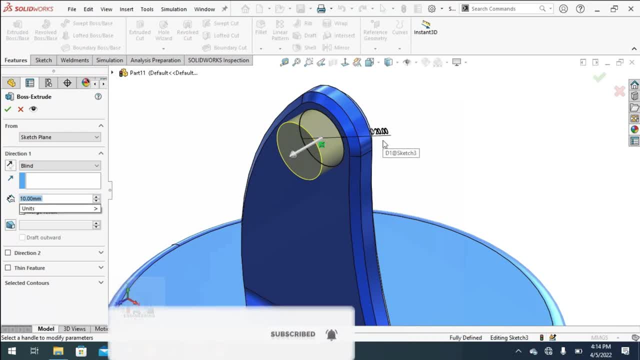 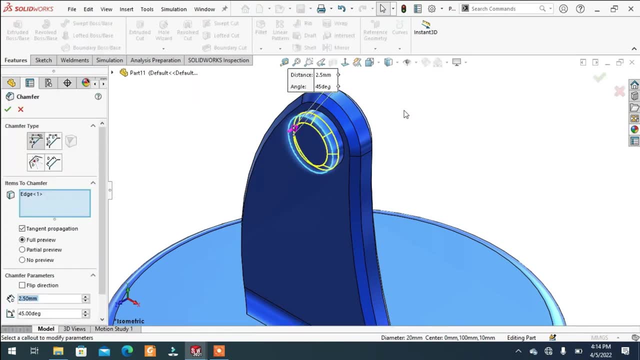 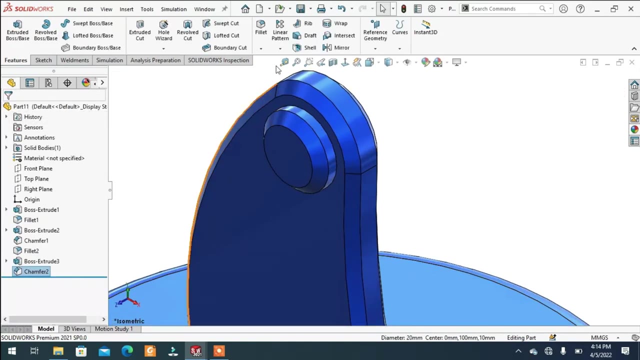 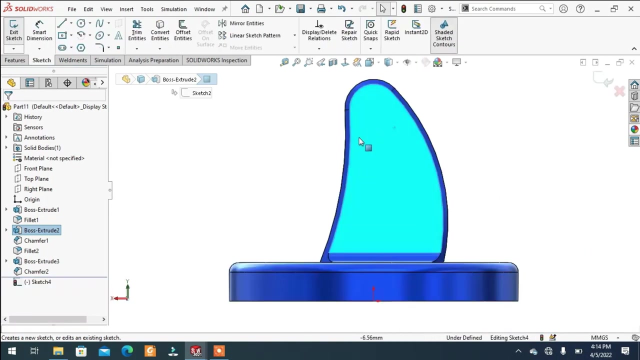 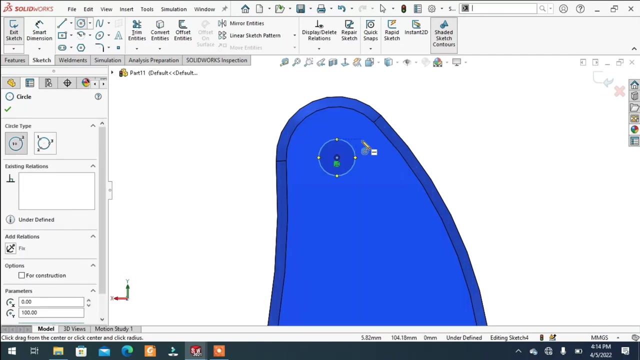 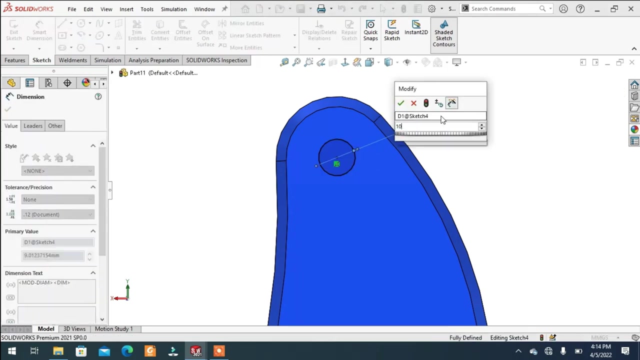 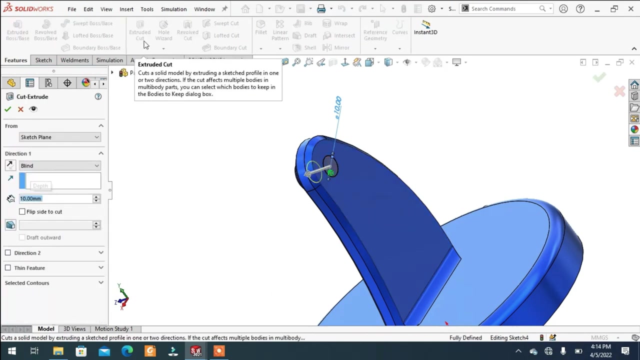 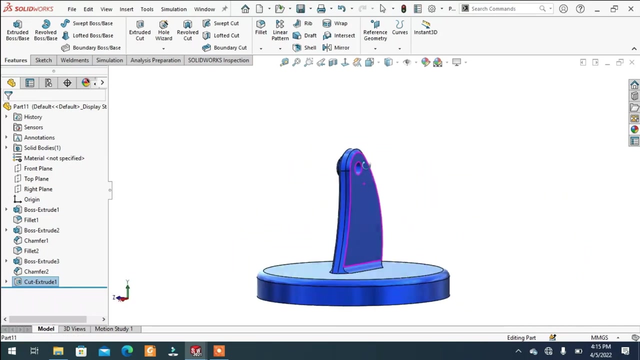 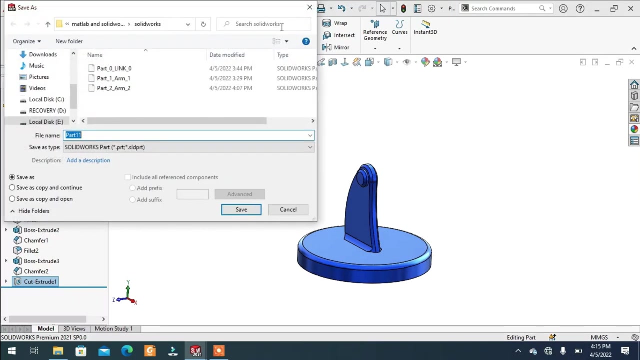 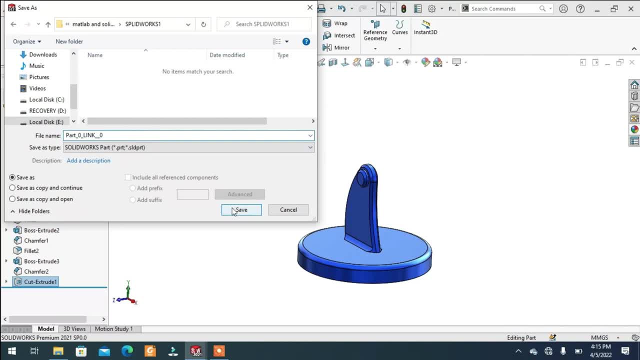 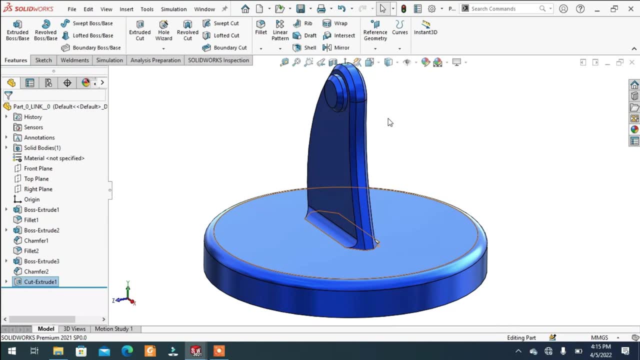 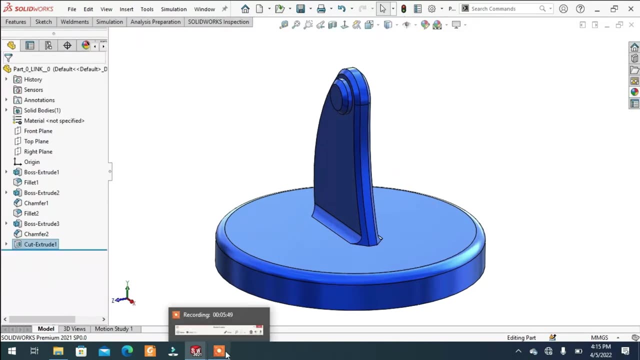 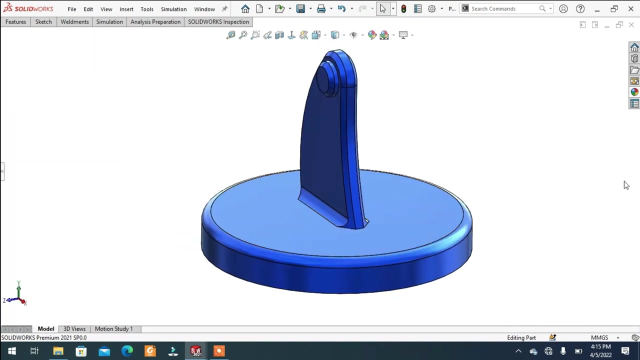 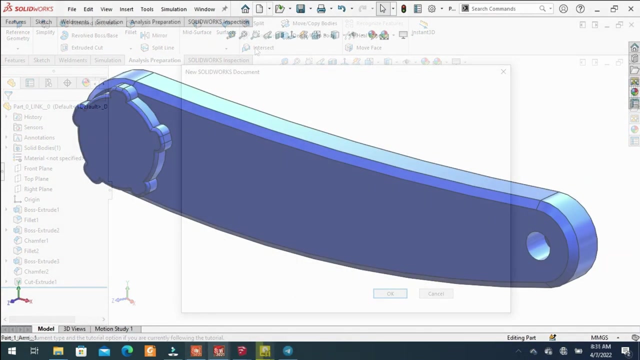 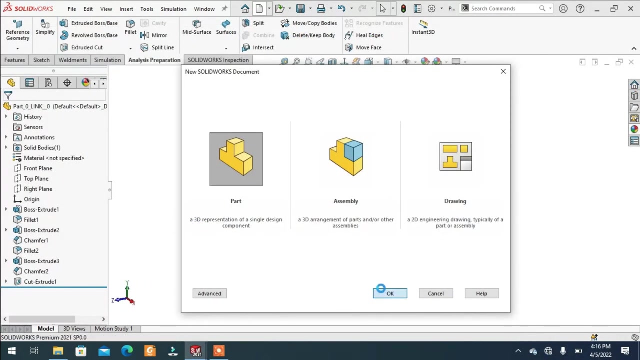 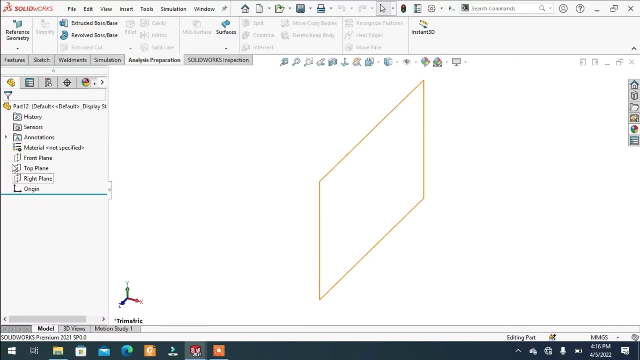 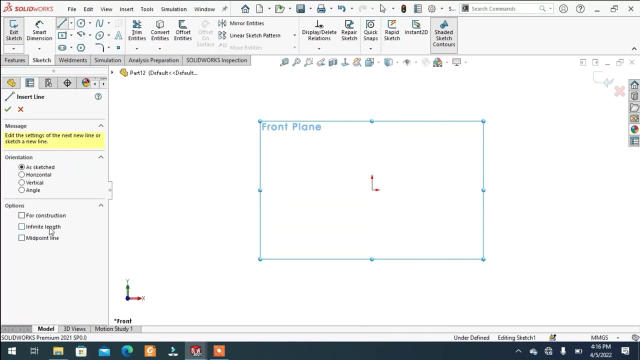 and make sure there is no gap between the the borders. open new parts and we will make the second part to start. open new parts and choose front plane and sketch, choose a midpoint line and if you select this midpoint you will drag it on the both sides and you can escape this and define. 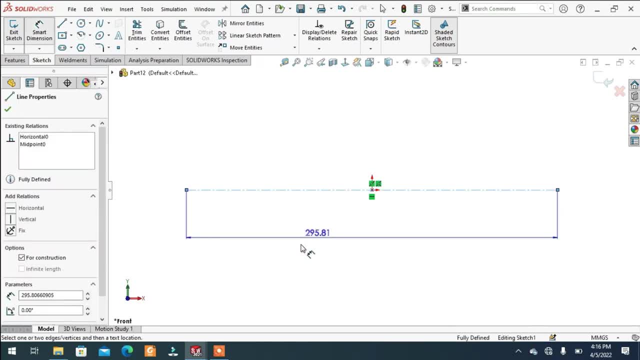 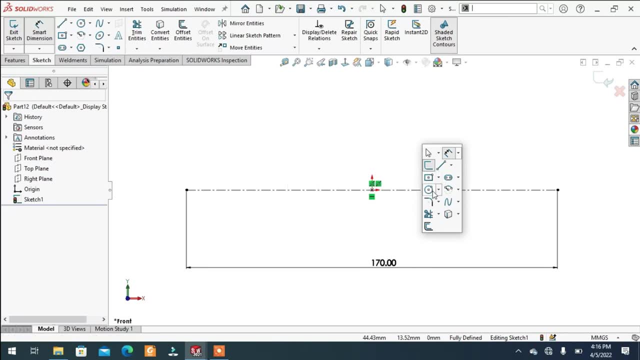 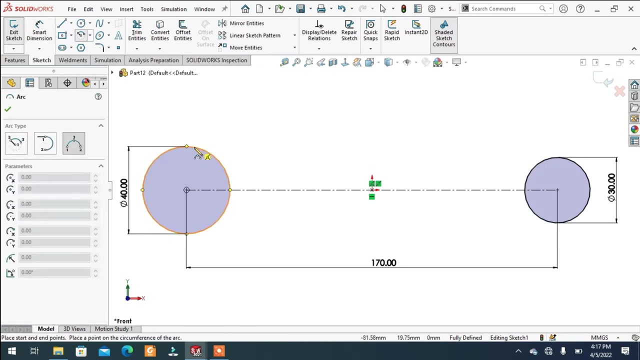 the length of this line and draw the circles, define the diameter of the circles and to connect this, choose three-point arc and select those two lines and one on the empty space and you can have this beautiful arc and make sure this arc is connected tangentially with the circle. 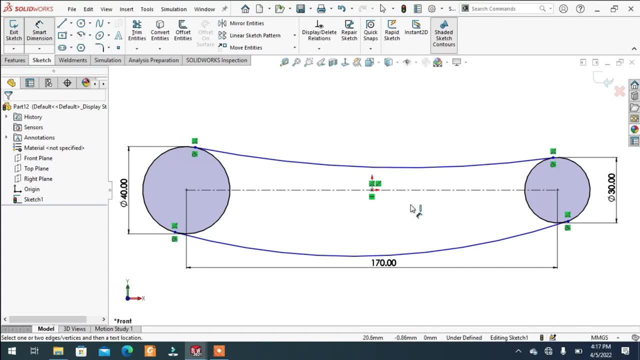 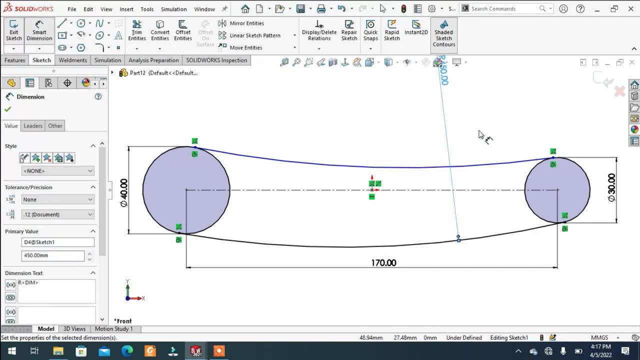 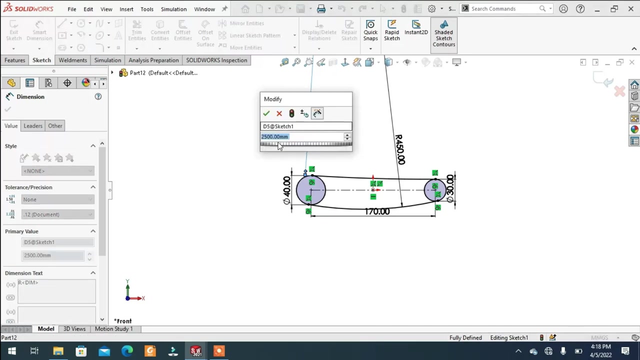 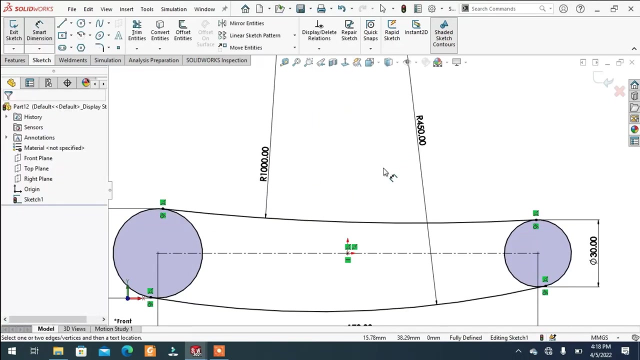 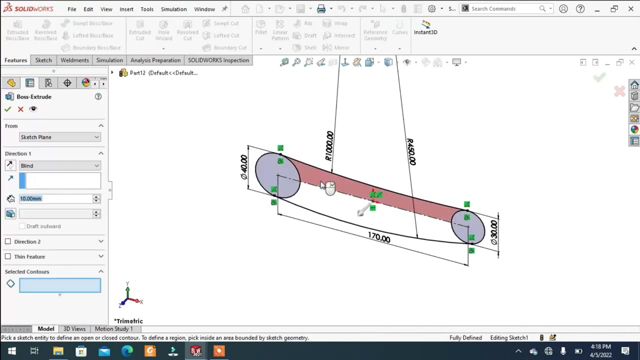 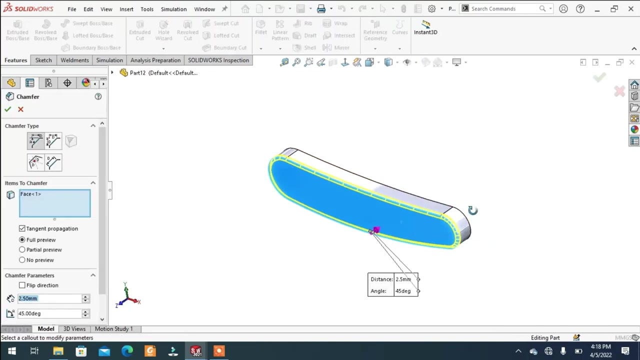 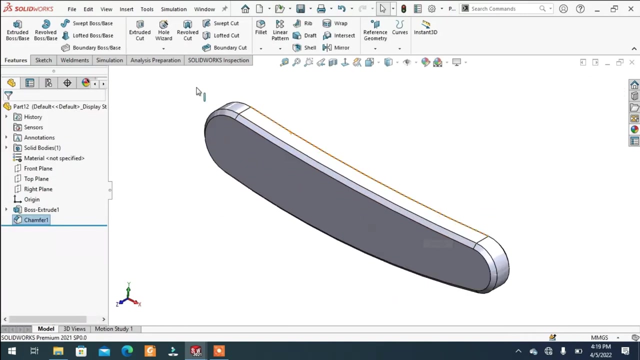 and define the arc radius and you can extrude it, select every boundaries and make sure you open mid plane and set the extrusion 15 millimeter and select this face and you can have a chamfer on both sides and click OK and we can also add some feature for better look on the face, on this face, so that you 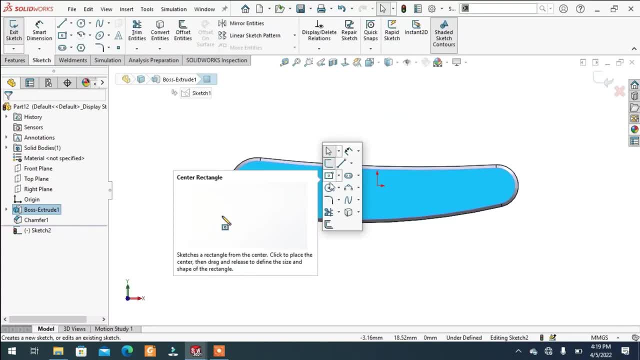 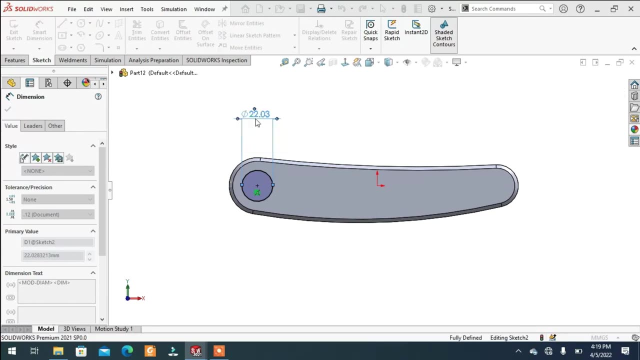 can sketch on it, we can change its height if you leave it as it is, and we can move the circle to the right and down just a little bit and make sure you get the correct angle. and in the next video we will add the circle and the visible part on this faces. 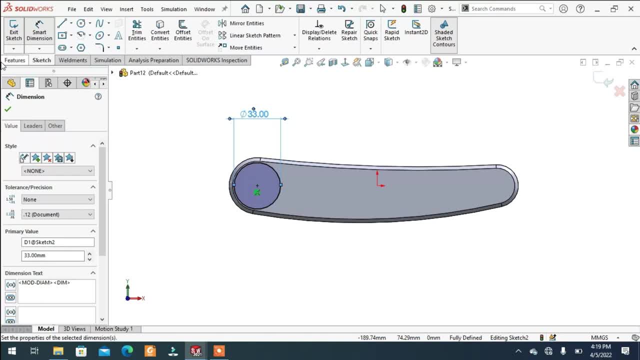 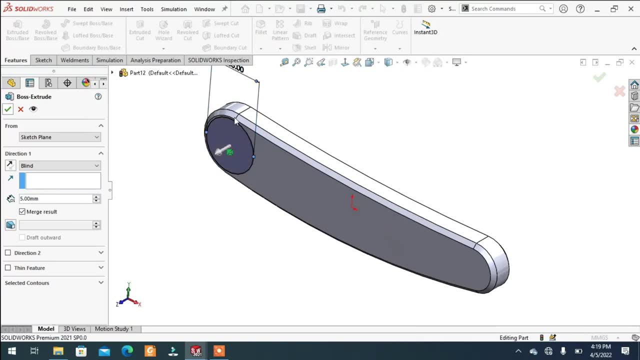 and we will also add some features on the right side of the face and the initial line of the cube that we will be adding to the right side of the face. then extrude this five millimeter and by removing the edge of the circle we can select the center of the circle and then we can start to create the circle and 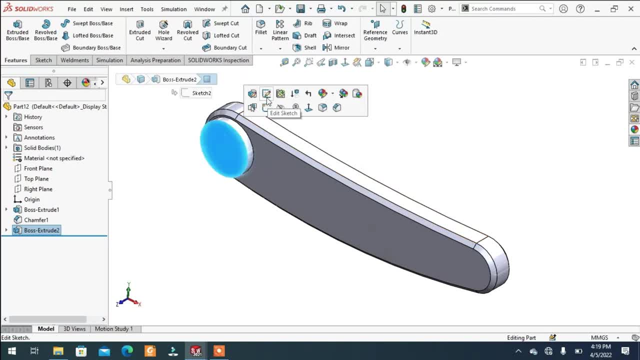 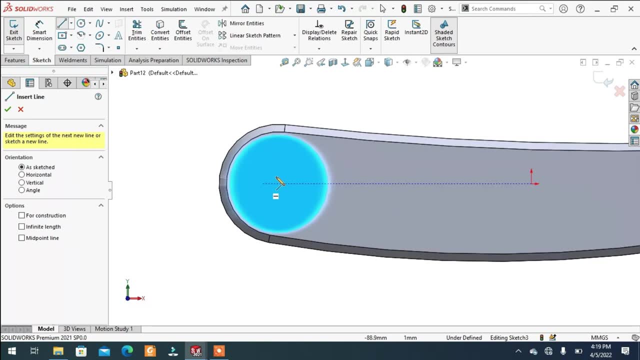 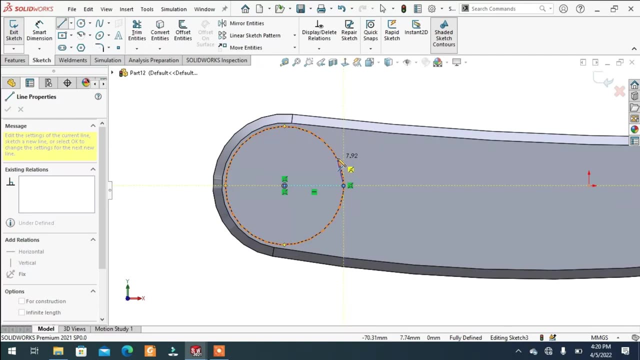 some components from this, we can have a better look of the hour. so, okay, making the center line as a construction line and drag this line and connect it and make it a symmetric, and the angle between these two lines are 30 degree and this distance is 20. 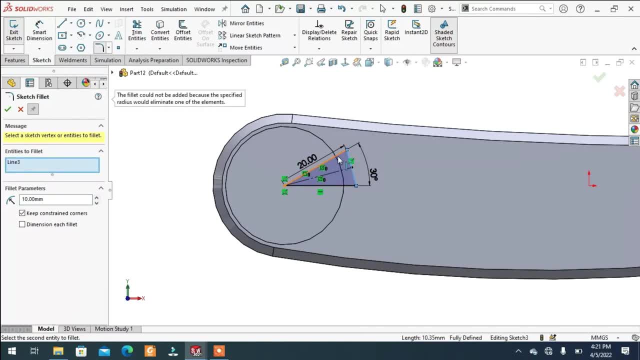 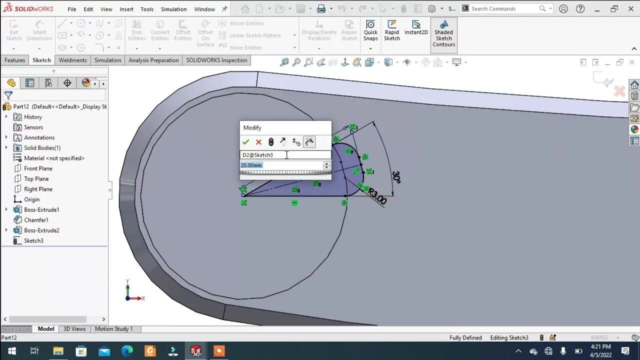 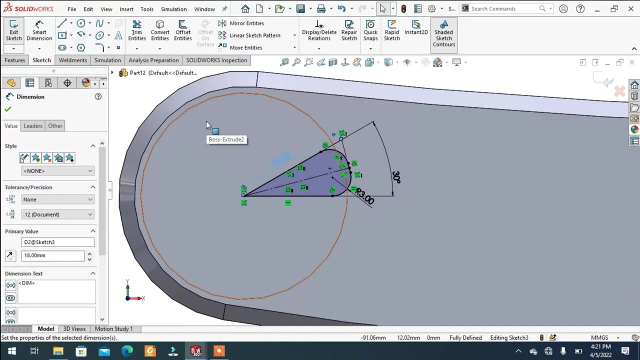 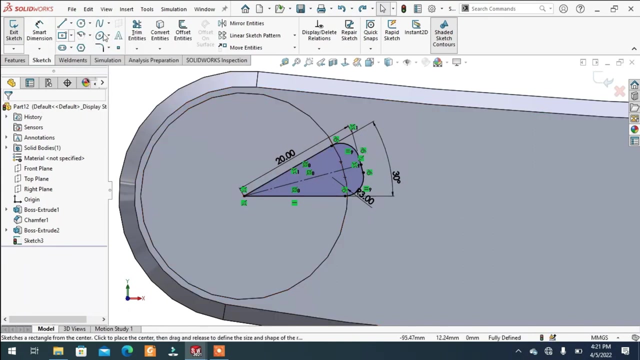 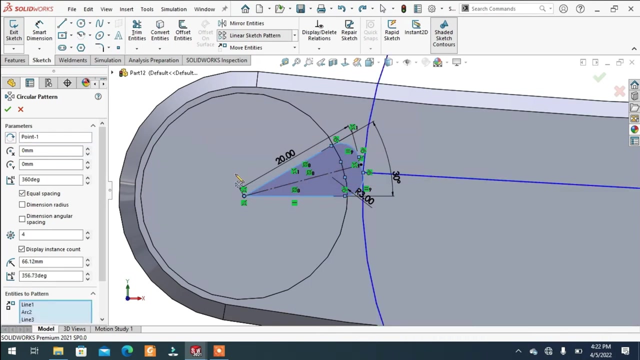 and reduce these fillets and select this edge and exit the fillet command. reduce a little bit and make it a little bit smaller and then you can have more. okay, undo this and just circular pattern and the axis of the pattern is on the center and entities to pattern is this sketch. choose this point. 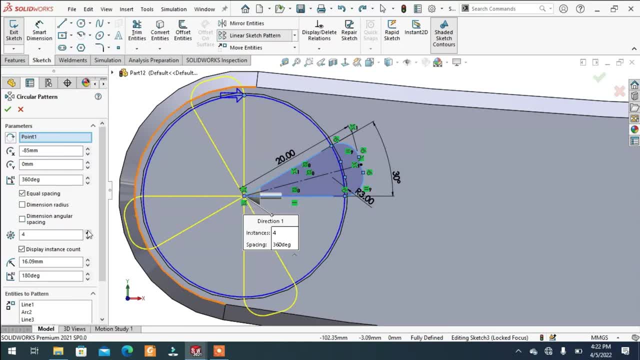 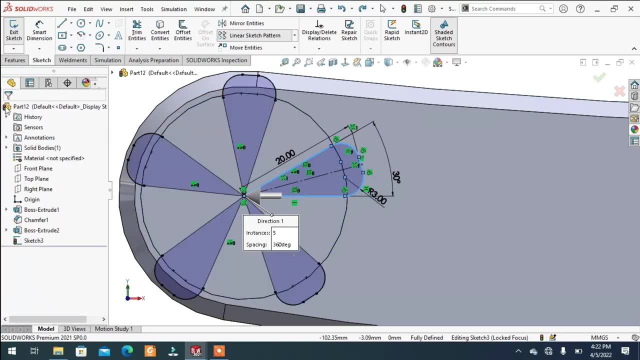 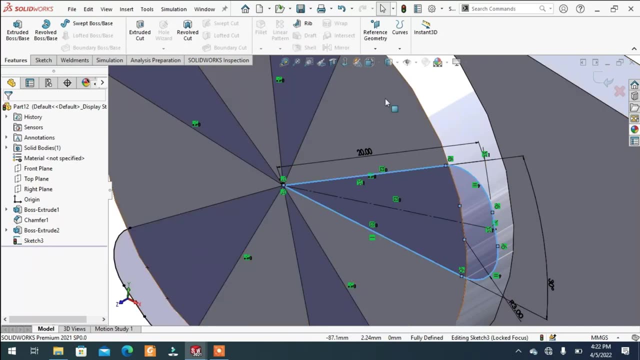 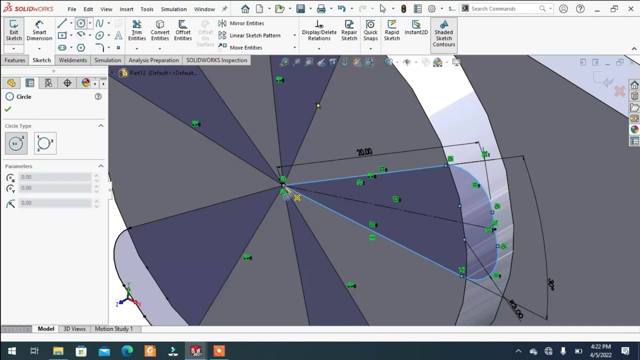 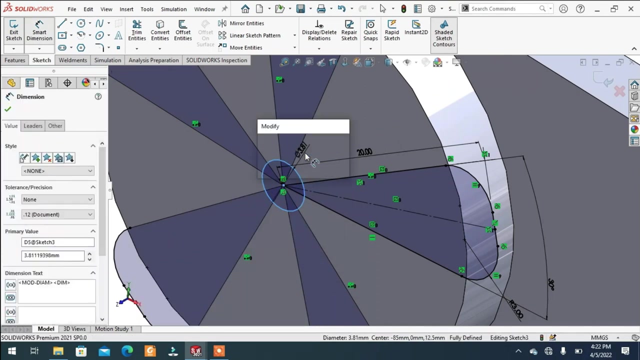 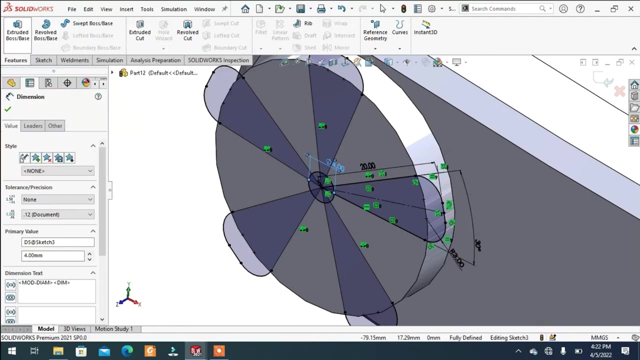 and choose a number of instances, how much we need this shape. I think it's low, it looks good and extrude this, since it is a vertex. at the end it will give us a near. so let's draw a circle with the diameter 4 and we can proceed. choose, extract both base. 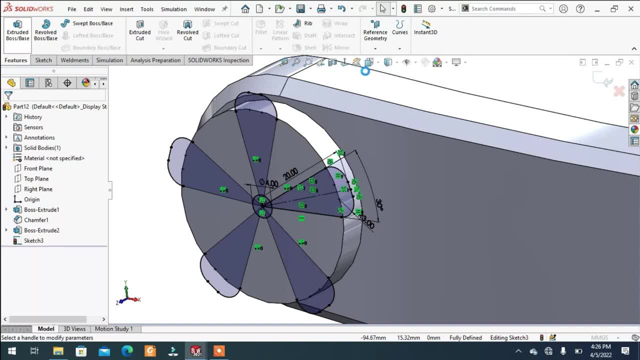 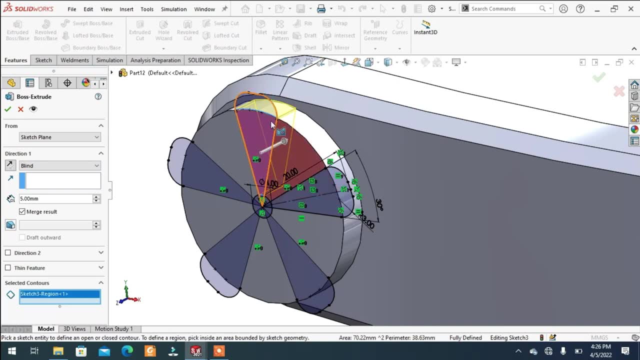 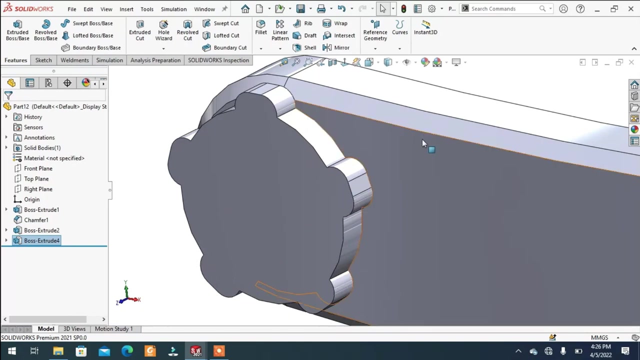 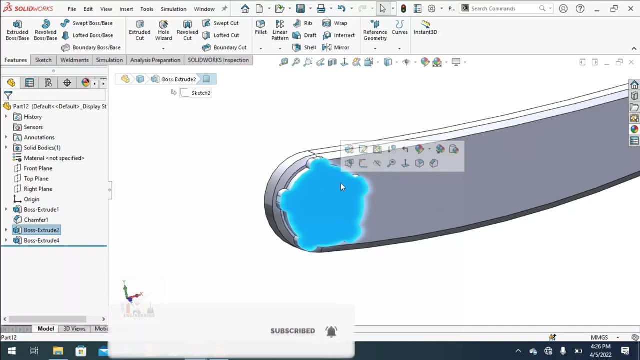 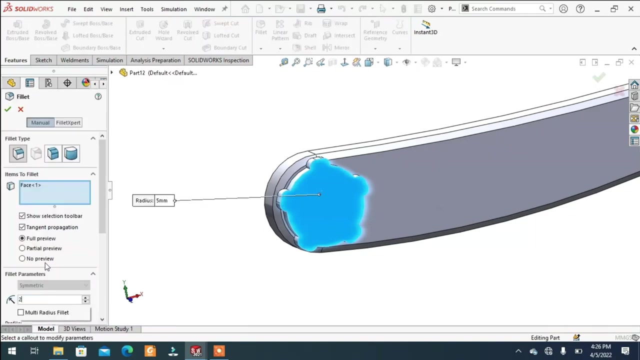 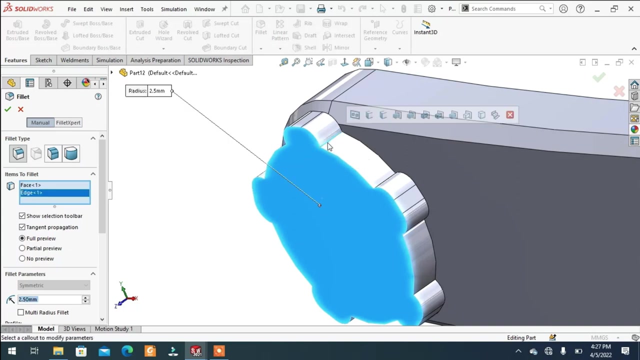 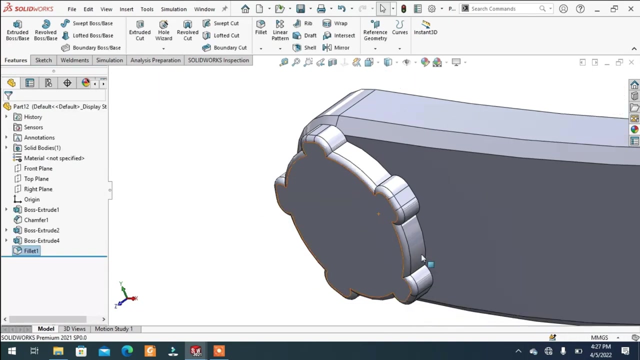 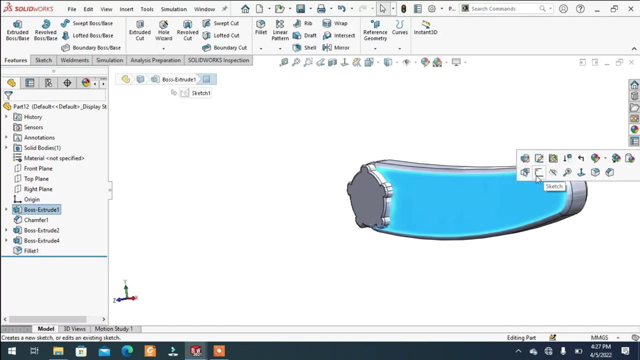 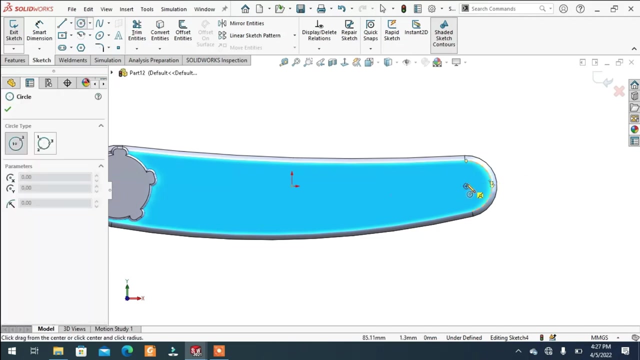 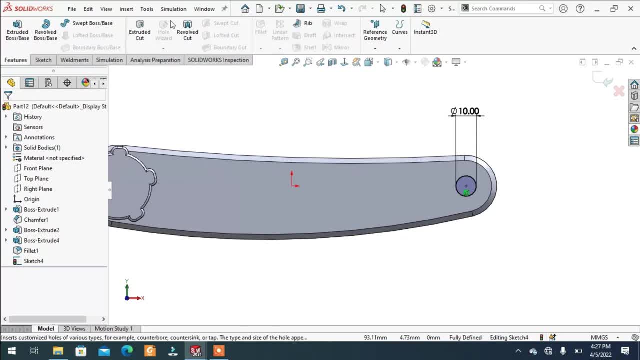 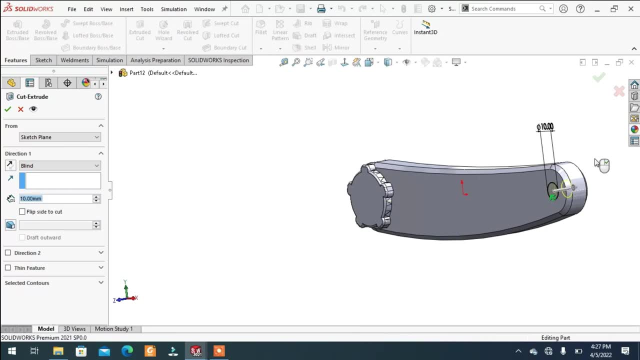 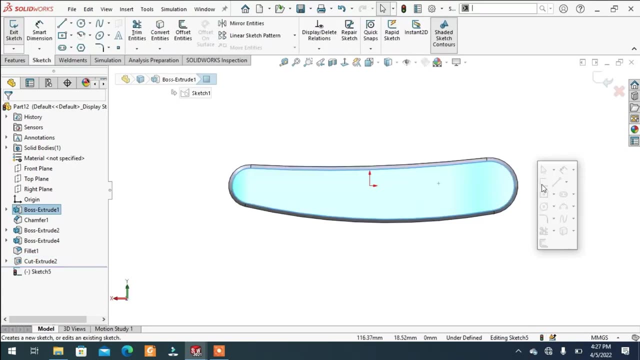 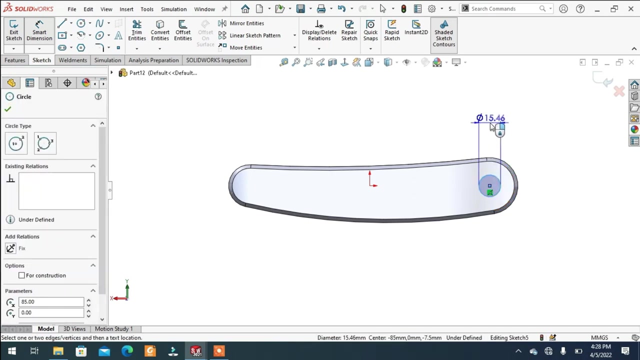 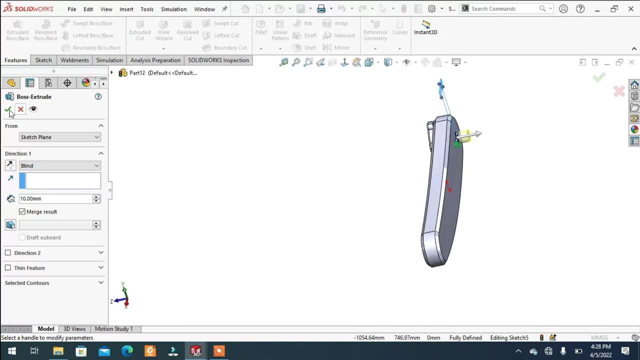 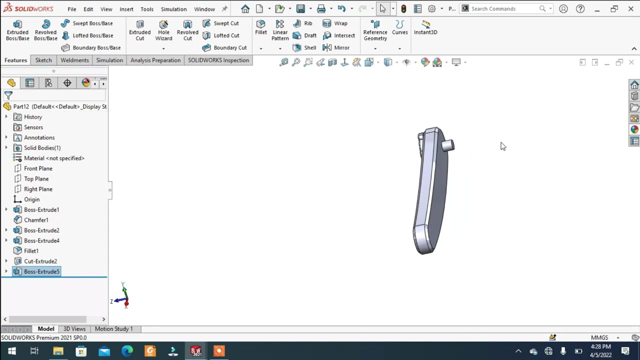 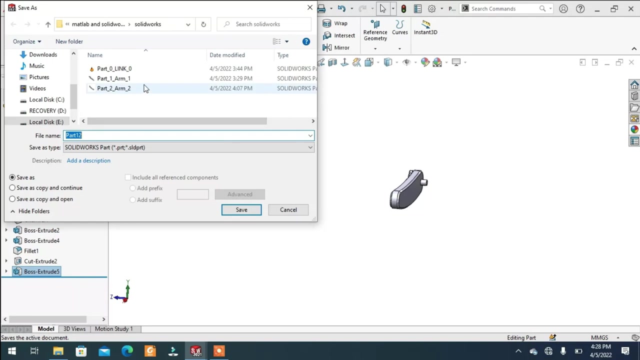 so so. so. so this cutout is used for connection of the pin from the next joint, and at the back face we draw a circle, set the diameter to 10 and and extrude both base. then we make this pin to connect from the previous hole, then save this next part again, make sure there is no space. 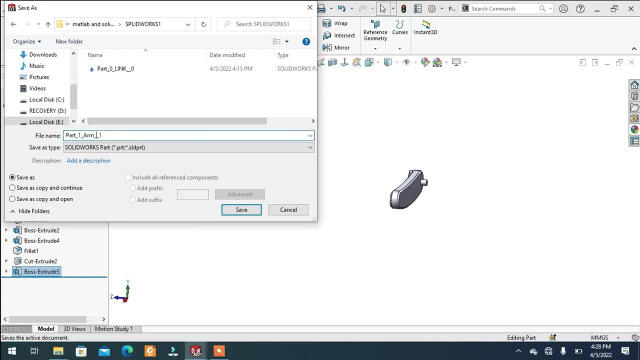 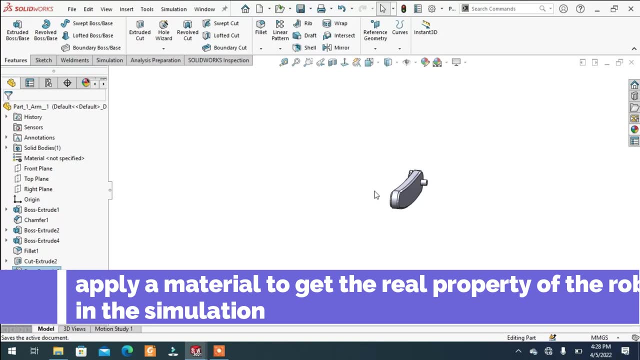 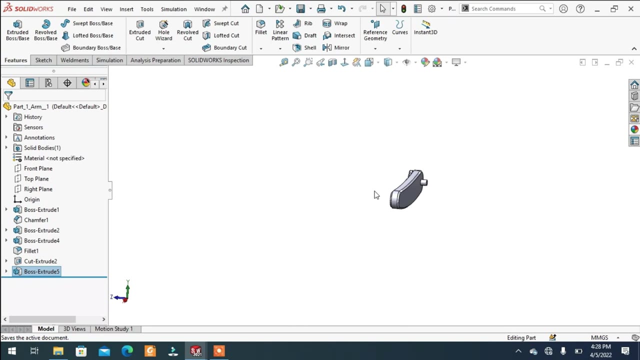 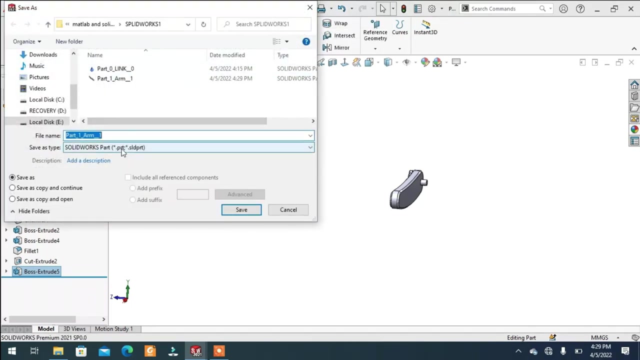 then save this next part again, make sure there is no space, then push onto the base after extension. if the part here for last, we import it and Europeans right, because it's going to be we project called subtype 4s, we name it asاشdj keinen sch乐. 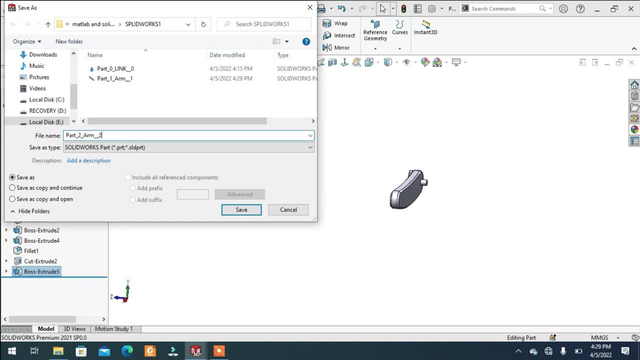 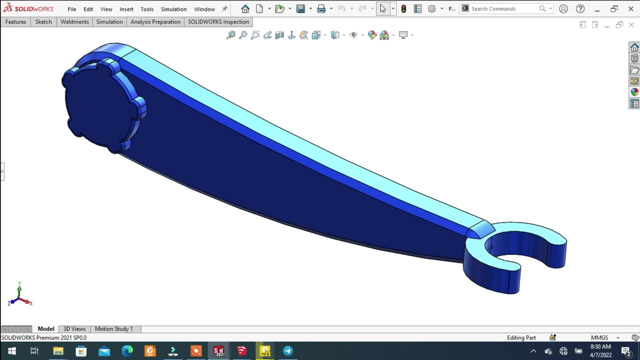 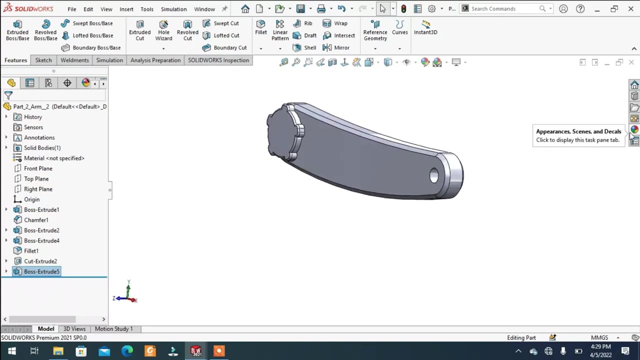 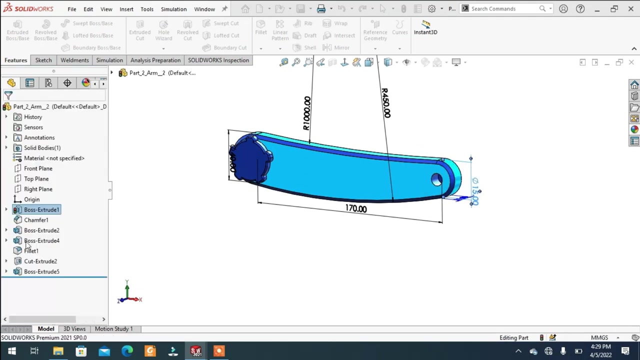 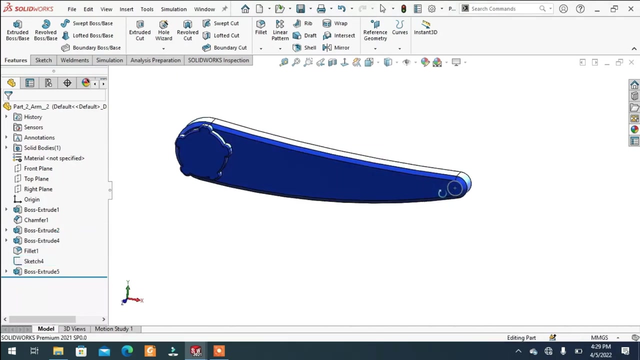 arm too. it looks similar, a little bit different. apply some appearance. then we can edit on this graphics area. double click on it and type 15 millimeter and, as you see from the design tree we can delete some components. I cut extra feature and also this sketch and this looks like it now. 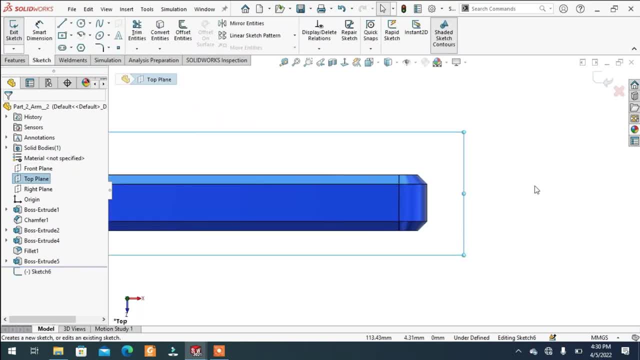 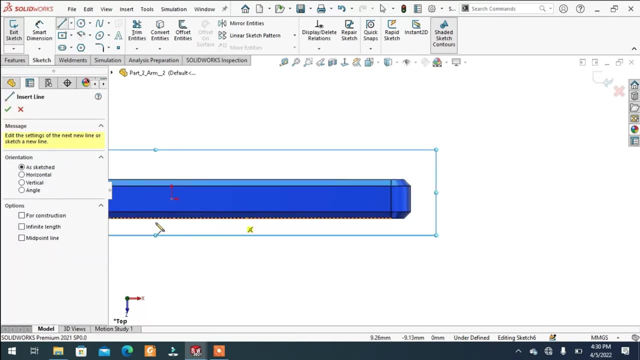 we will draw a creeper like structure just to mimic the creeper. it is not a real one. if you want to make a real gripper, I have made a video. you can also find the link in the description box below. you can also find the link in the description. 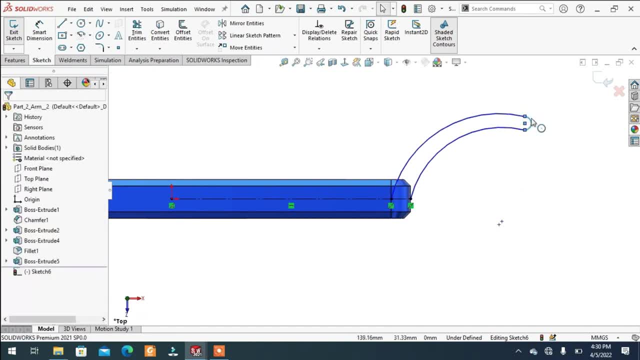 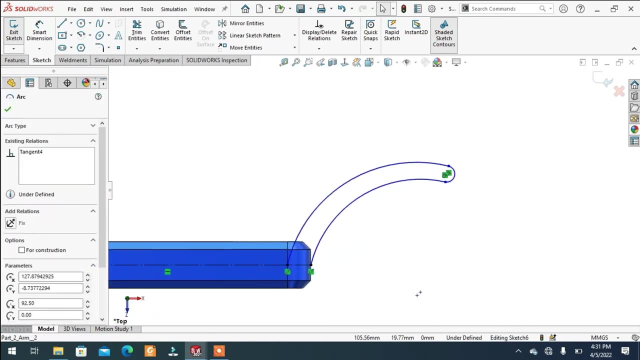 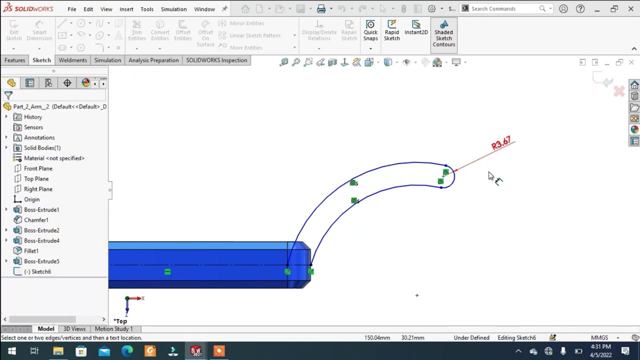 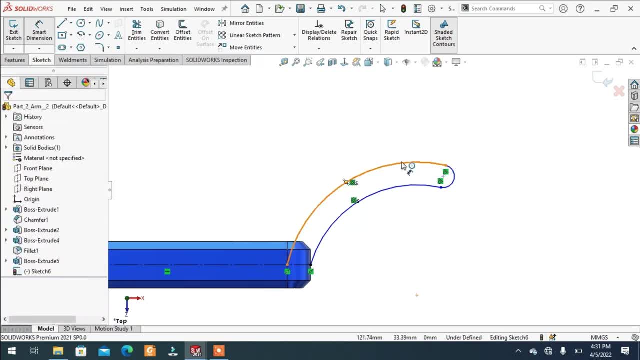 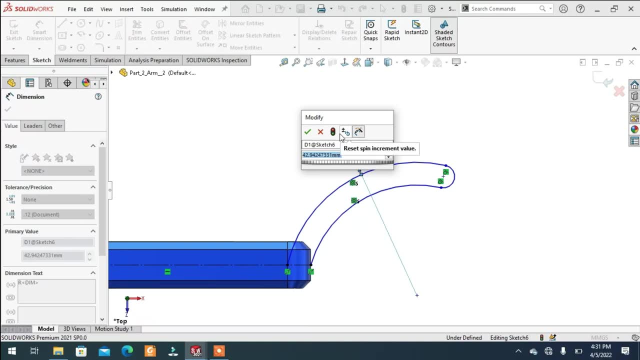 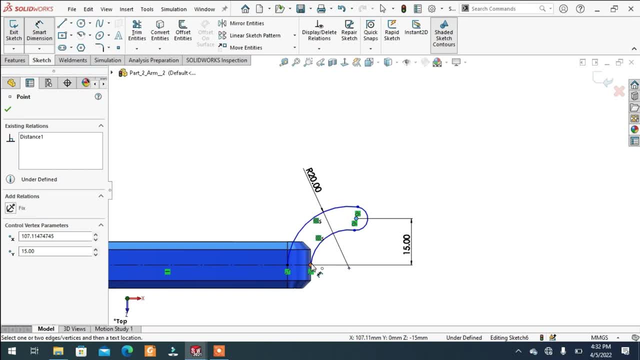 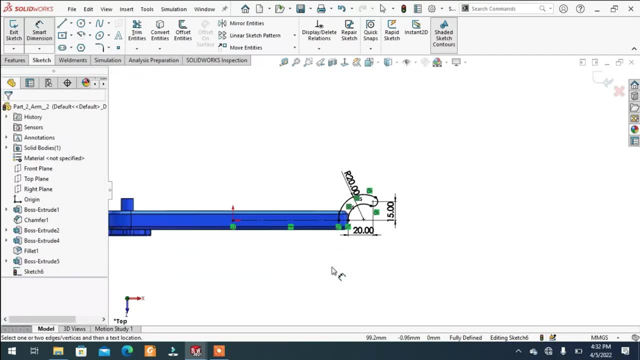 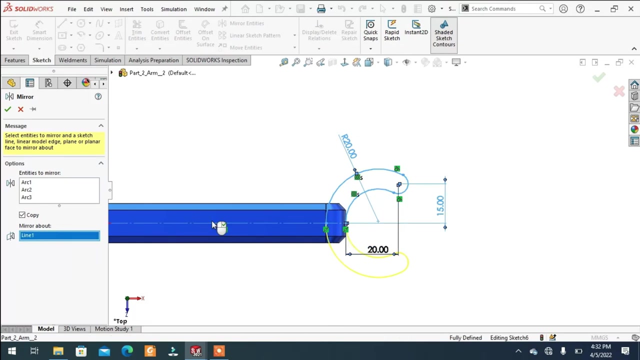 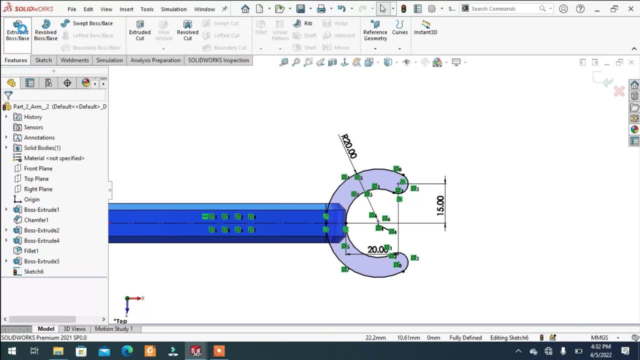 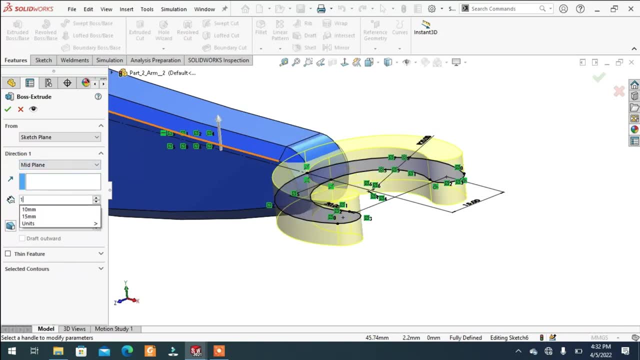 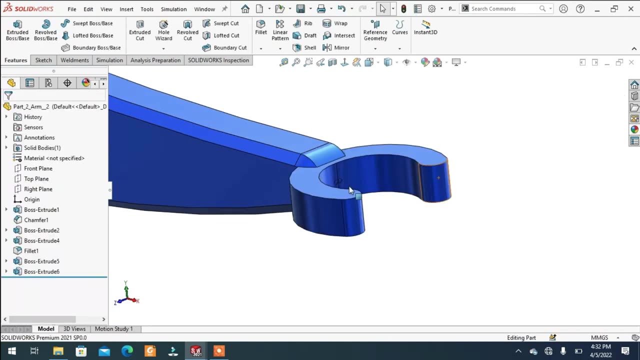 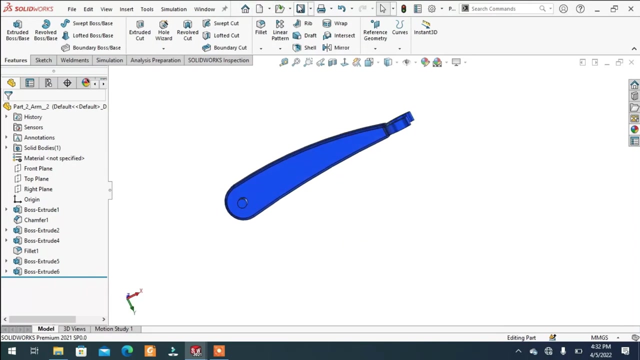 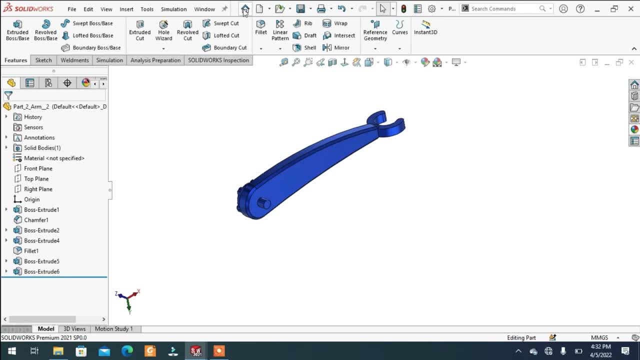 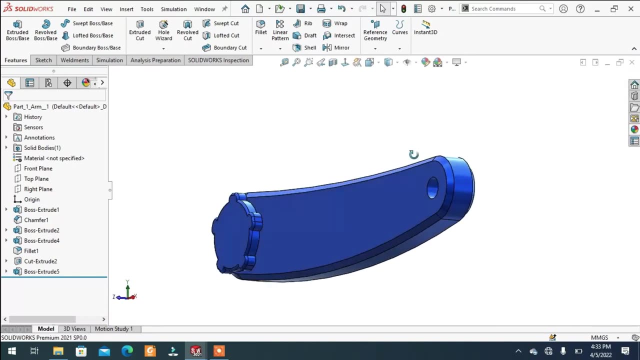 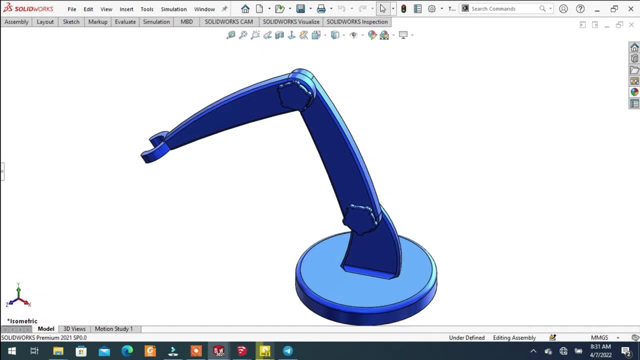 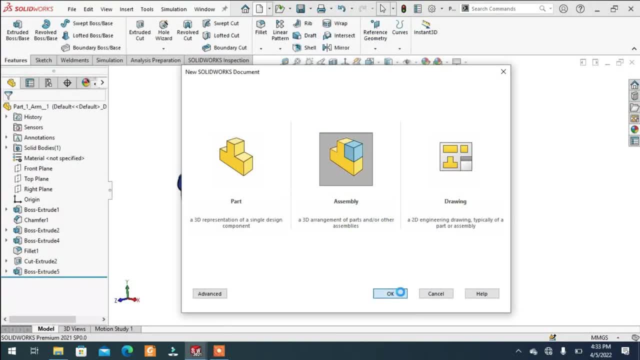 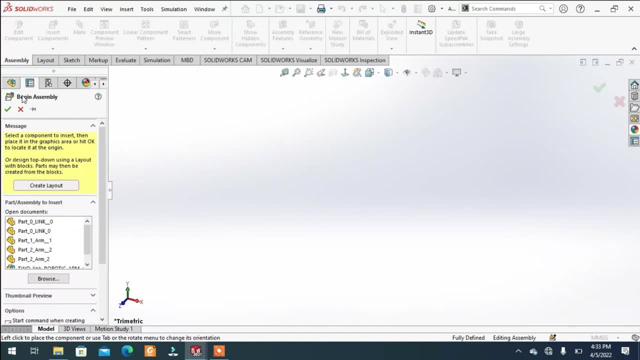 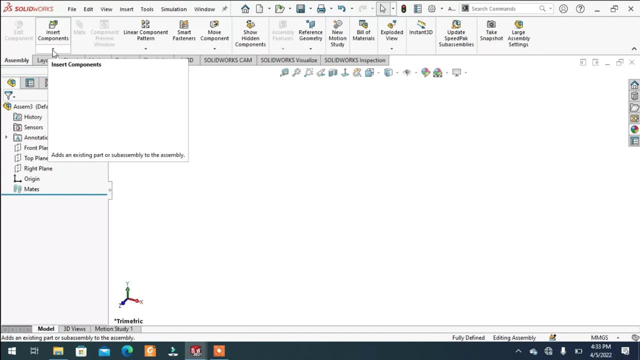 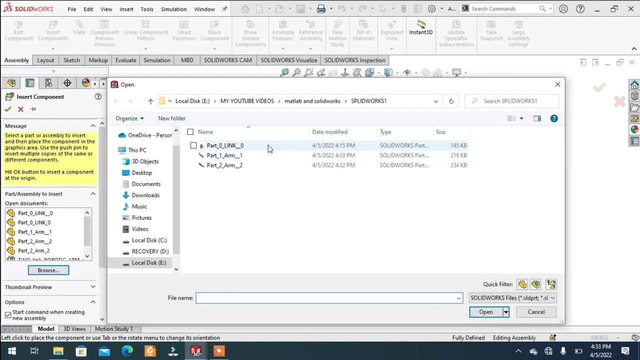 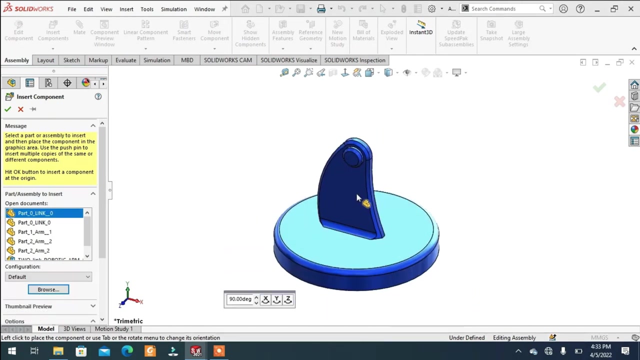 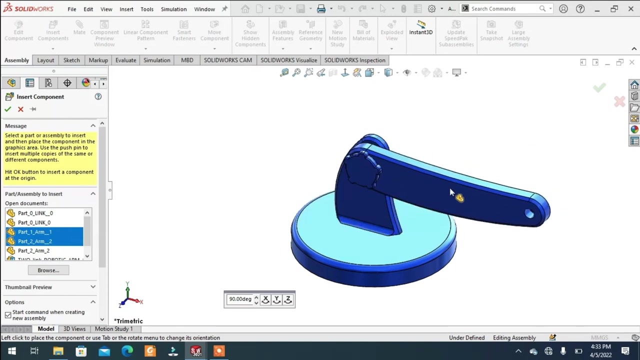 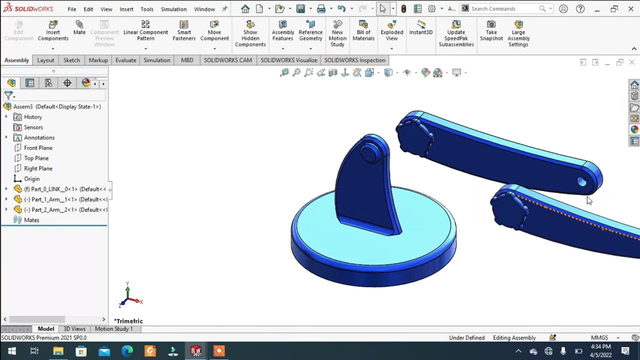 unidentified lines. unidentified lines- unidentified lines. first, open the assembly and make sure it's in whites and insert this components and choose the first one, the link zero, and place it around here and similarly, insert some components, the arm one and arm two, place it anywhere and okay, the next one is we have to assemble this. now. the parts are imported. 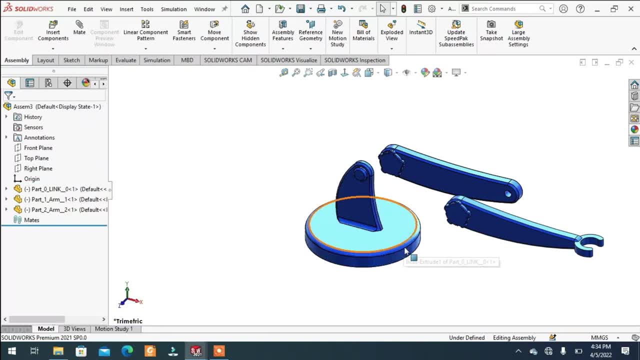 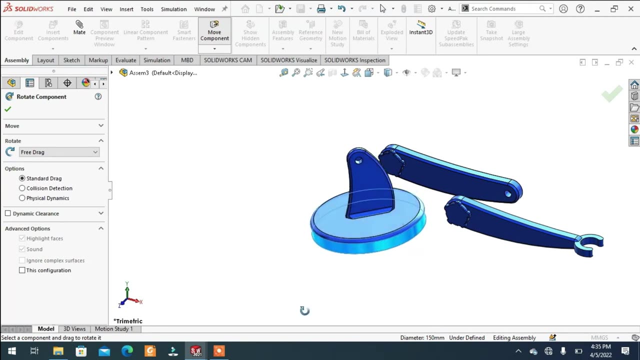 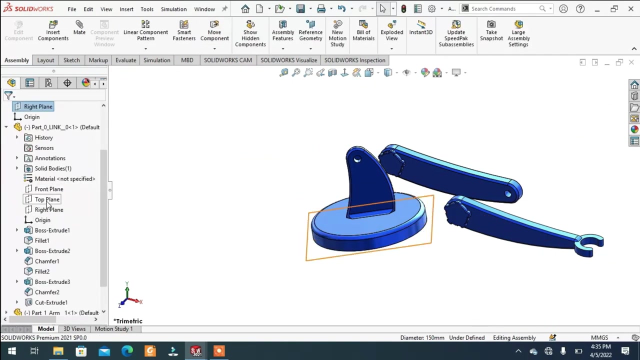 make sure this first link is float to better move, for proper visualization, and i think it is good position and let's make this top plane to the top plane and we can fix it now. as you see, the coincidence is gray down so that we can delete it. 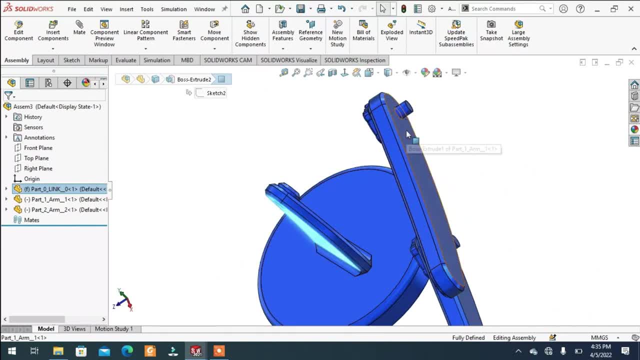 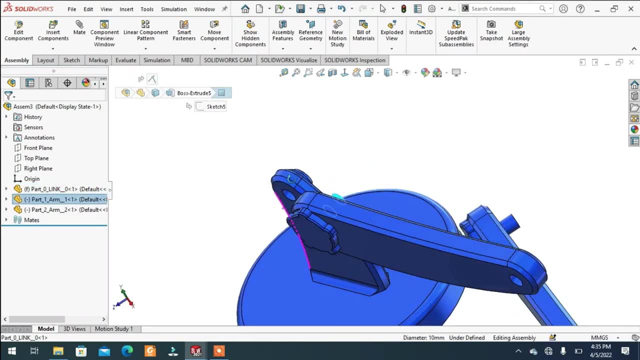 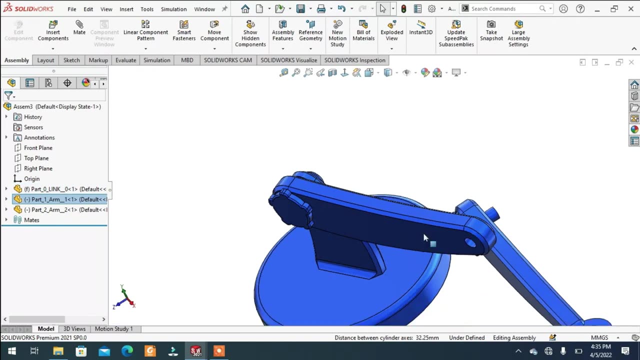 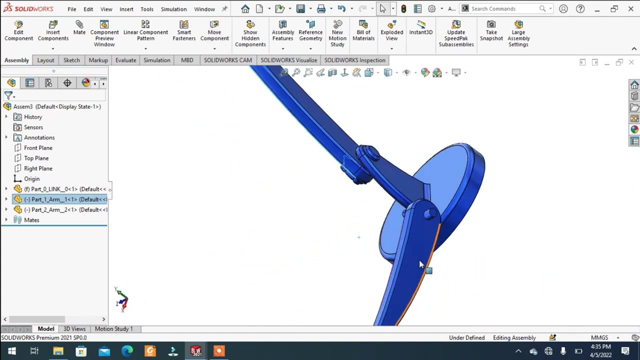 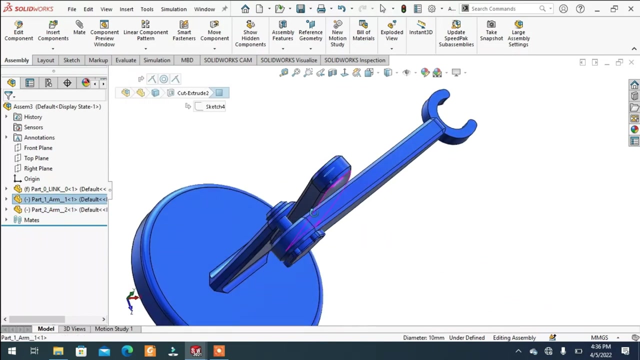 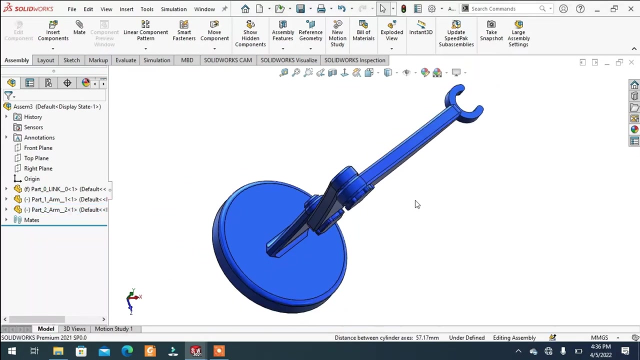 and choose those faces and make it coincidence. choose this circle and in the inside circle, make it concentric mix. then this will act like this: it will be coincident with that. and similarly, drag this and select this circle and this one, make coincident smiths. so these myths will work. this coincidence mates will work. 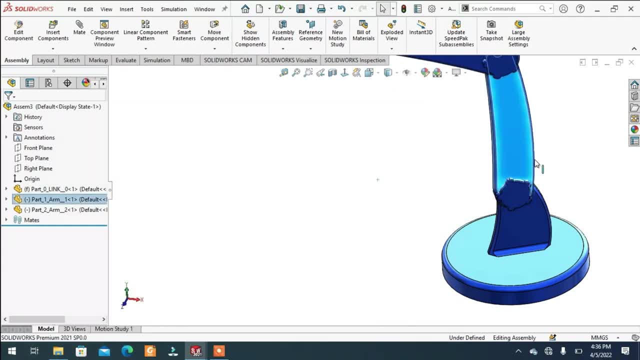 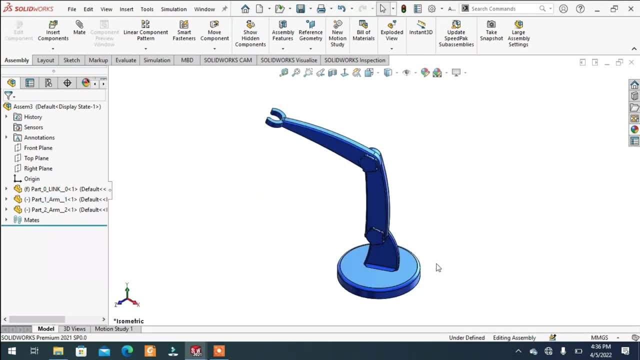 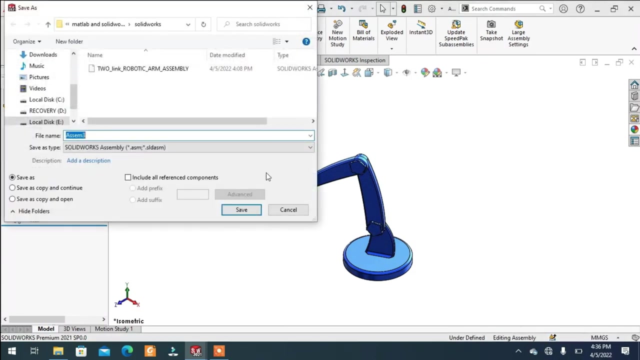 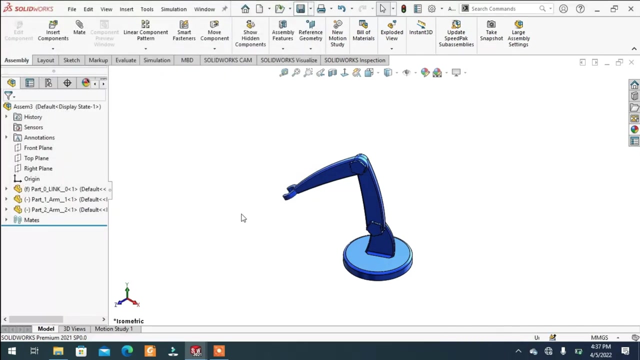 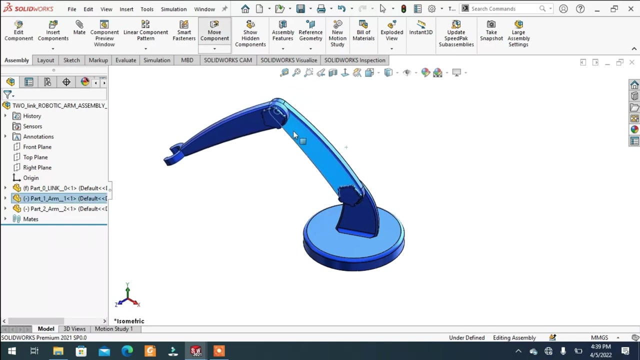 on the matlab as a revolute joint for other projects. make sure you select the appropriate mids for exports, since every type of mids are not supported in Simulink, and save these robots as this name. okay, the robot mechanical module is now finished. the assembly is finished, so. 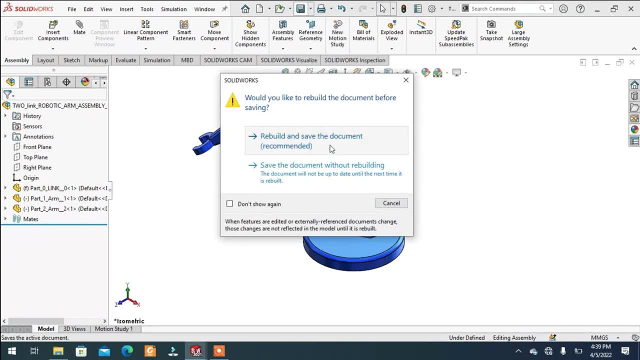 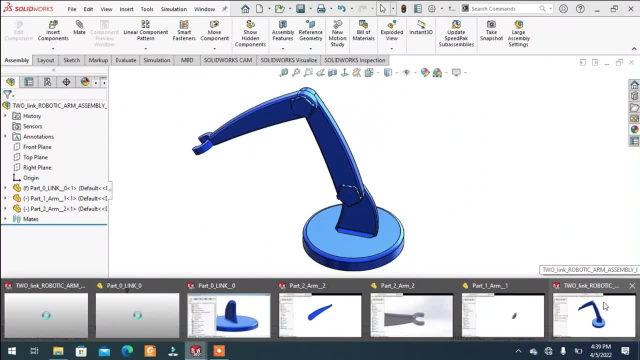 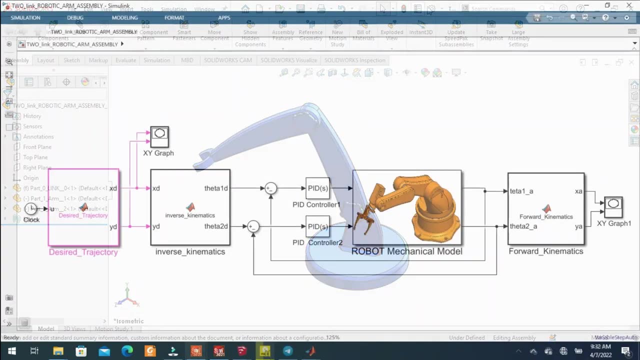 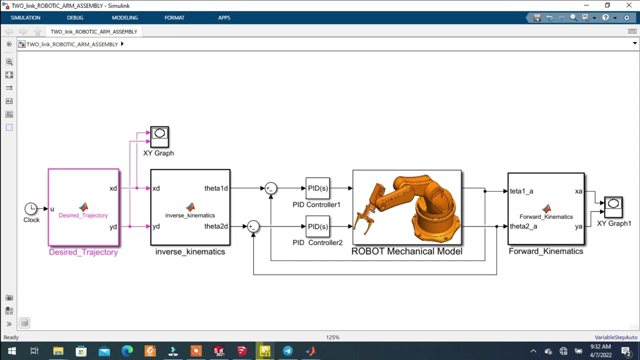 that we can proceed: the MATLAB run the MATLAB as an administrator to call. when we export the SOLDOCS model into MATLAB, we can call the MATLAB. before I start an in-depth explanation and modeling of the control algorithm, let me give you a brief overview of the projects that we are going to do up next. 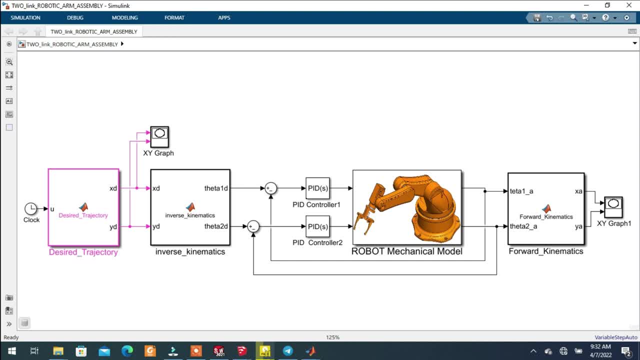 as you can see from the control diagram, there is a clock signal that help us give a time variable to determine the desire trajectory of our robot in time. The desired trajectory is in a plane, since it is a planar robot, so it gives us two variables as an output: xd and yd, As you. 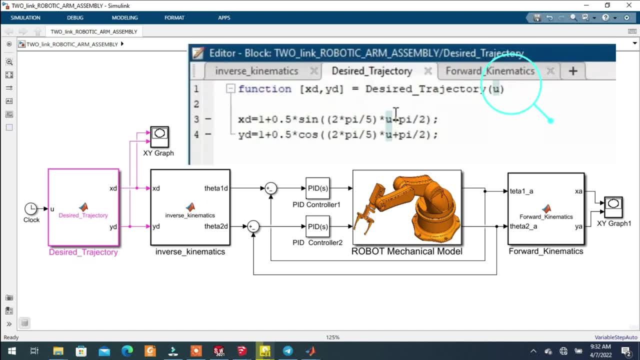 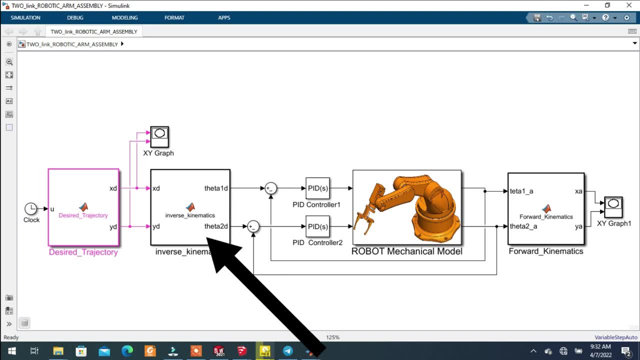 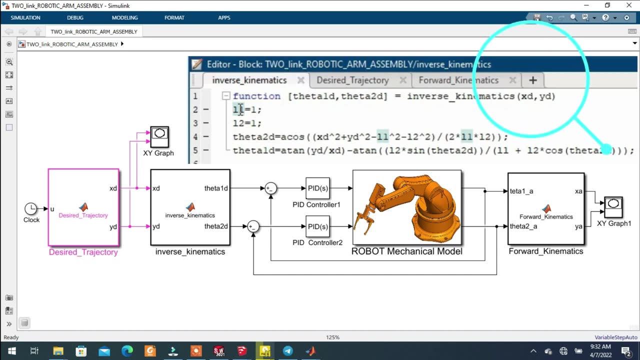 can see from the code, both variables have the same input, u, which is the clock time that we have seen, And the next one is the inverse kinematics block that takes the desired robot trajectory xd and yd and gives us an angular position of the robot to follow its trajectory with, respective time, The 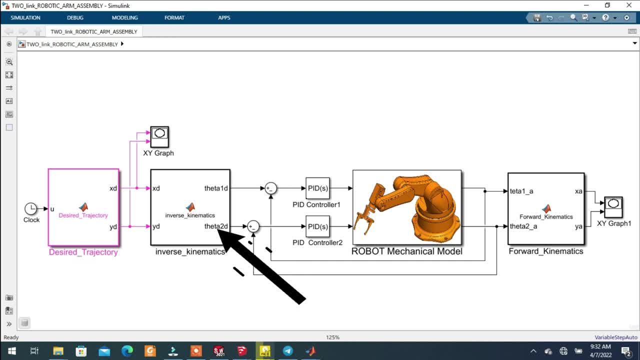 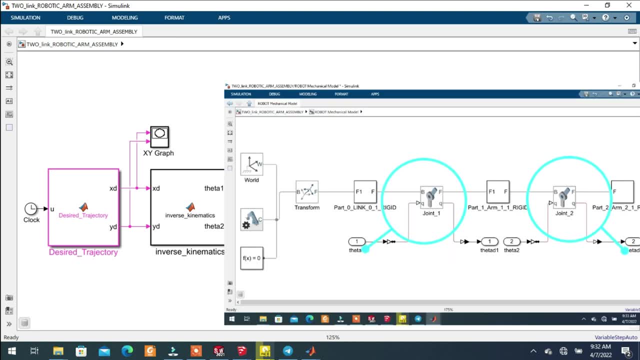 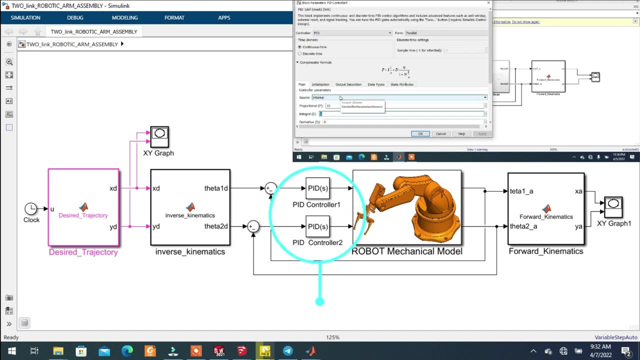 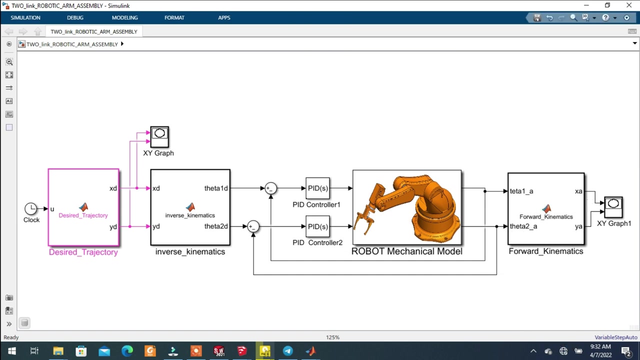 angular positions are θ1 and θ2, and these two angular positions are actuated by a motor, either by a stepper motor or a servo that needs to be controlled using a controller. In this case, we will use use a PID controller and that will text the error signal and tries to eliminate it to. 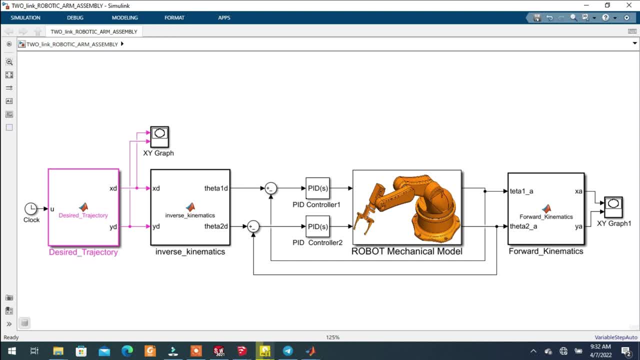 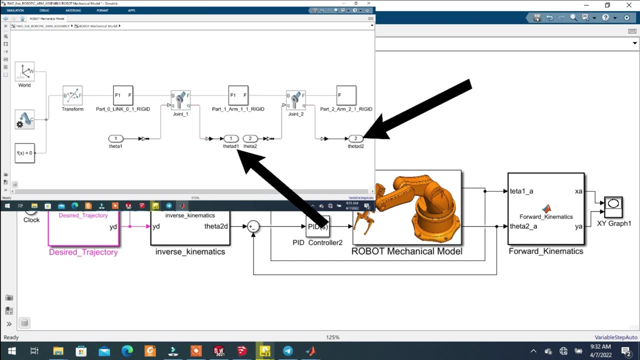 get the desired trajectory the same as an actual trajectory. The error signal is created by subtracting the desired angular position of the robot, which is the output of the actual motor from the robot mechanical model, and the desired angular positions that come from the inverse kinematics block. 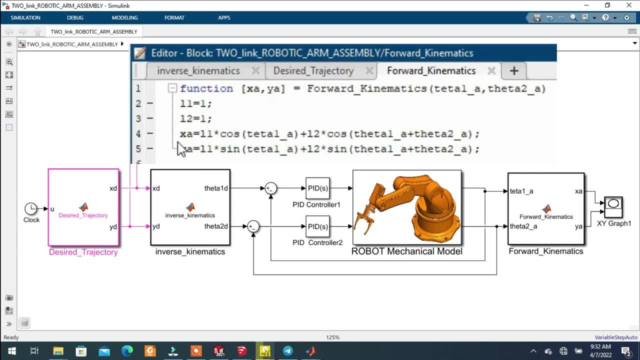 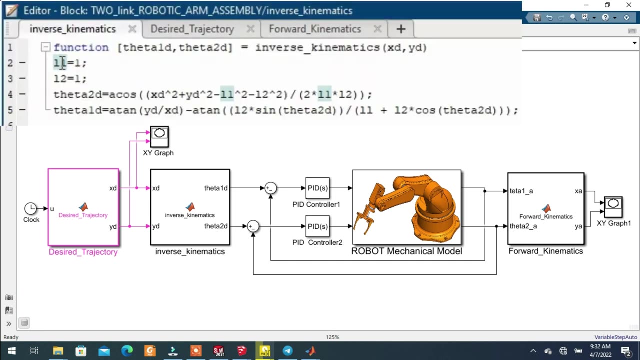 And the final block diagram is the forward kinematics block, which uses this just for visualization purpose. It takes the angular position of the robot and it gives us the position of the end-effector, of the robotic arm, with the respective of time. You may have been confused about how can I get the formulas that guide the robot like. 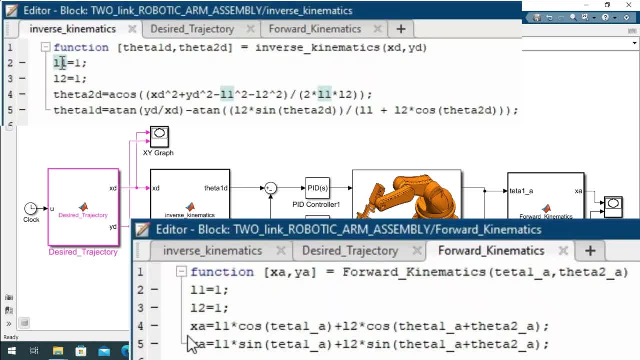 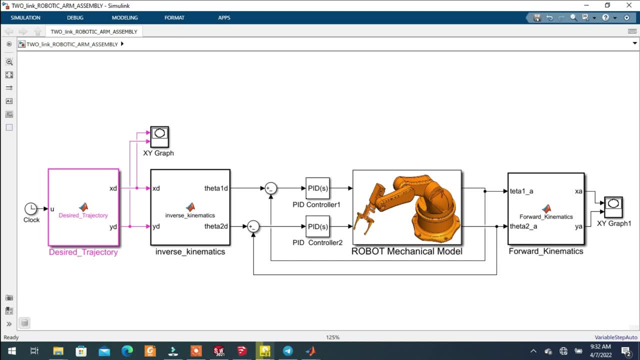 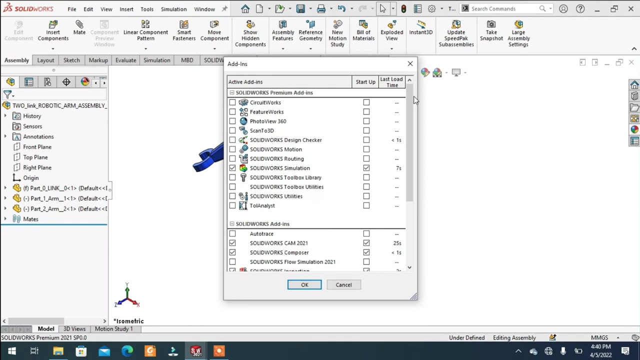 inverse kinematics block. I will give you an in-depth mathematical analysis to find its forward and inverse kinematics of this robot in a separate video. The link is in the description below. First, let's go to add-in and activate the simscape multibody link. 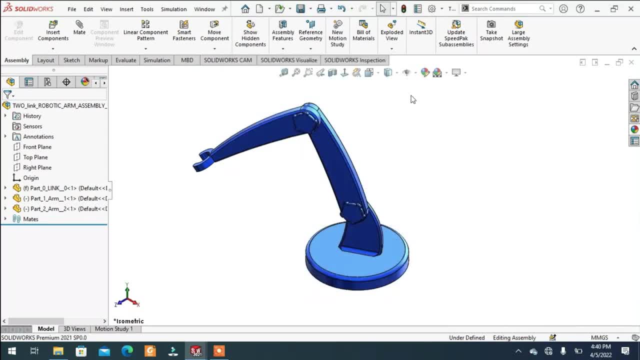 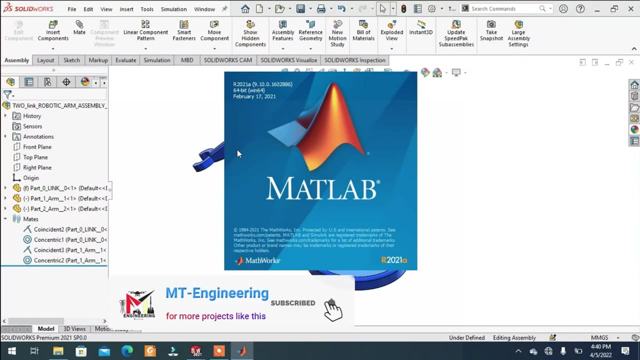 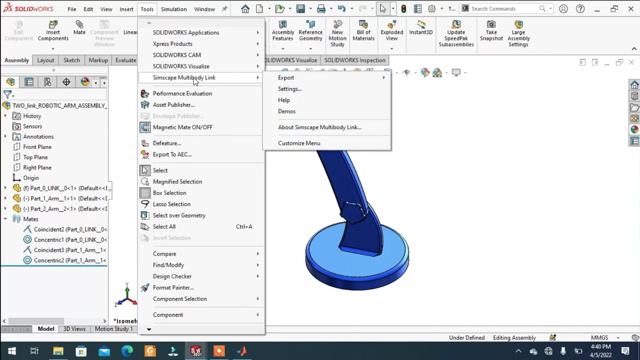 And after that we will check out our partners. The mates are only these four mates that guide the robots. And after we check this, the MATLAB is opened now and we go to tools and under tools, simscape multibody, and export, then export it as simscape multibody. 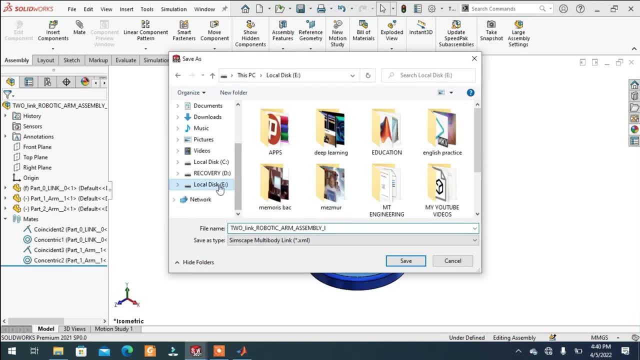 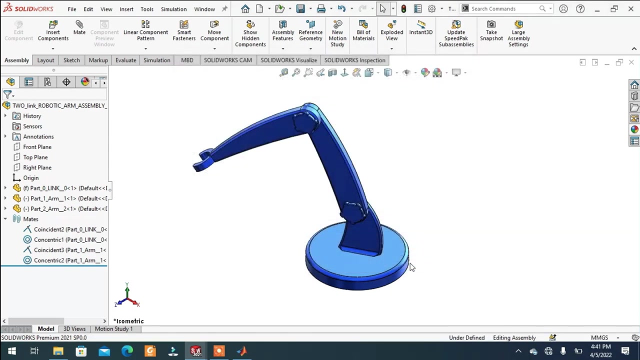 Then you can find your directory to save the XML file And this XML file will help this robot will hold this robot's properties. Make sure there is no space between the letters. Let's go to the next step. Let's go to the next step. 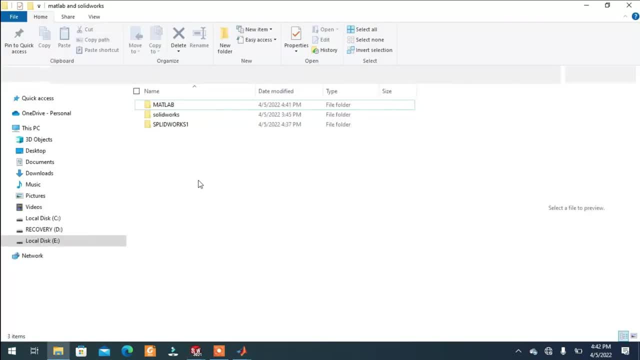 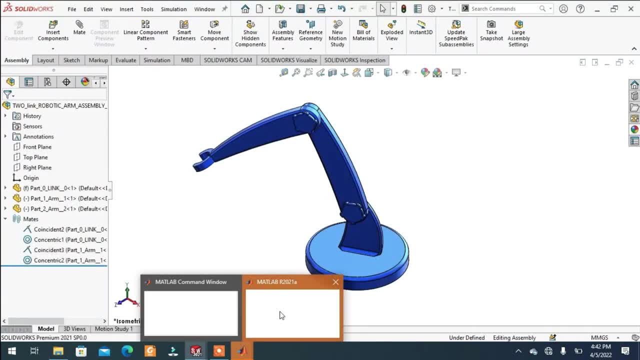 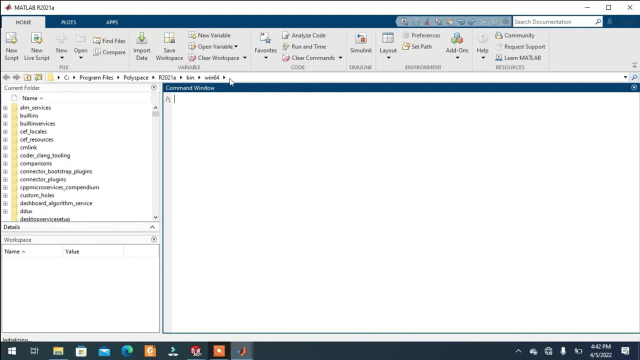 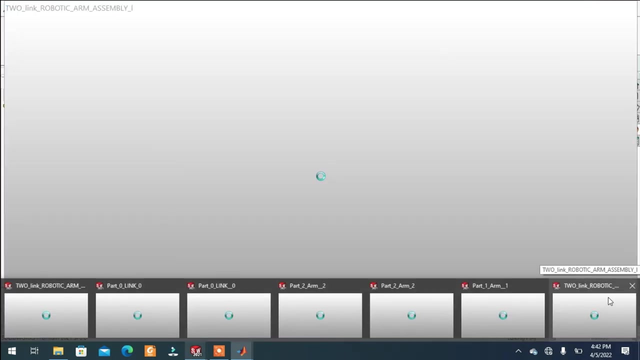 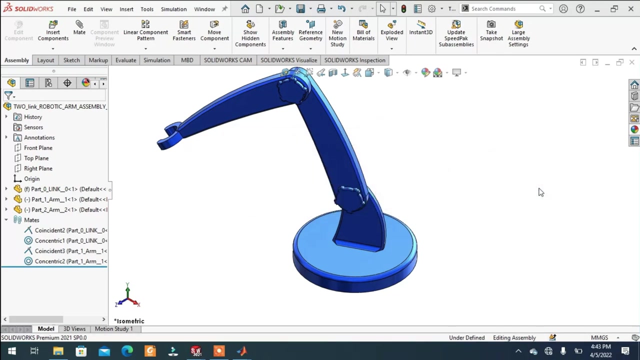 Let's copy it and paste on the MATLAB command window. under this bar we will paste the directory of our uh project. Okay, now, since we doesn't export the model still now, it is blank. okay, the process is now activated and, and after some time we finish the exports. then these are the 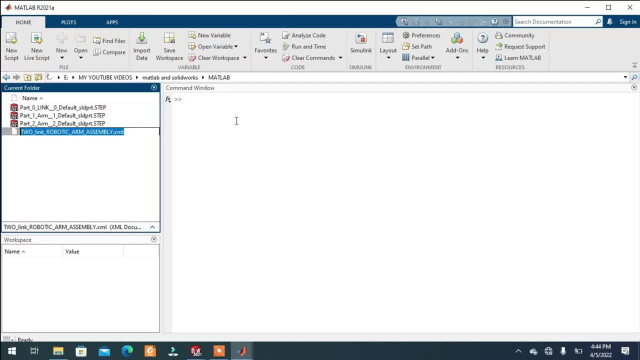 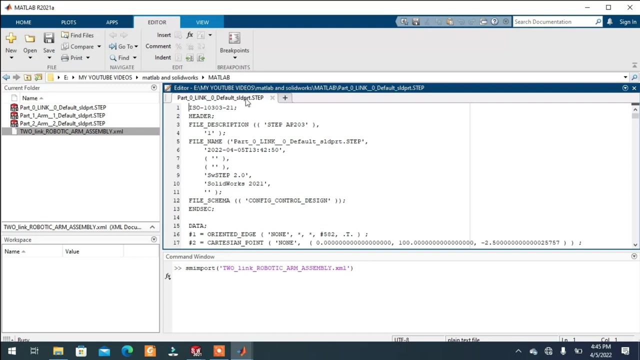 step files that holds the robots and the XML file. is that integrate those step files into some one components and we can import these step files into MATLAB simulink using sim imports command. then you you can copy and paste the name of your projects, then enter and after some time it will load. 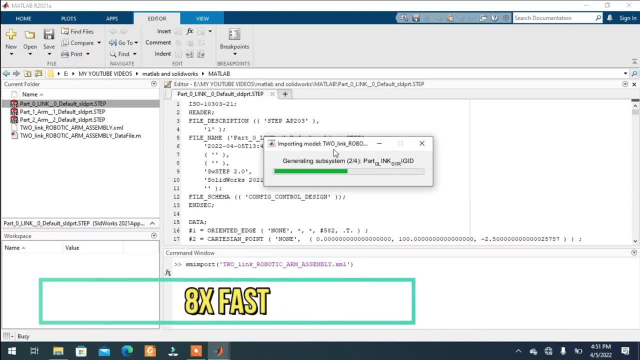 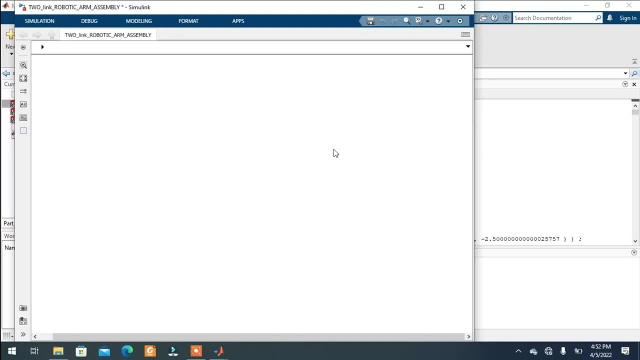 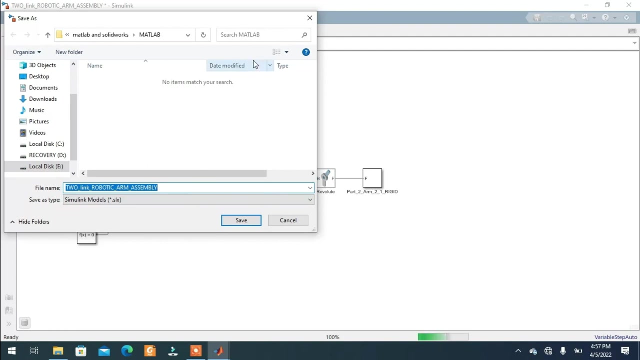 the robots model and it generates a simscape multi-body link or simscape multi-bodies. as you can see, this is a simscape model of simulink model of our robots. is that we have did using solders? then make sure you save this file again. 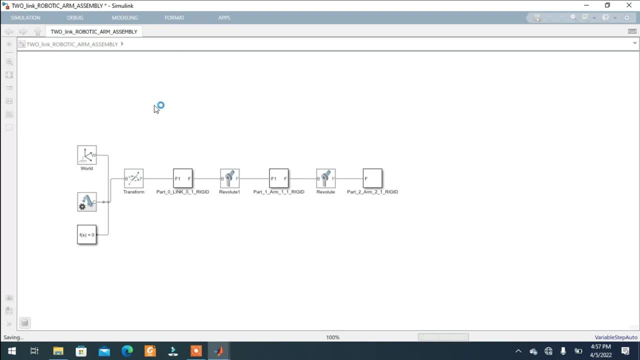 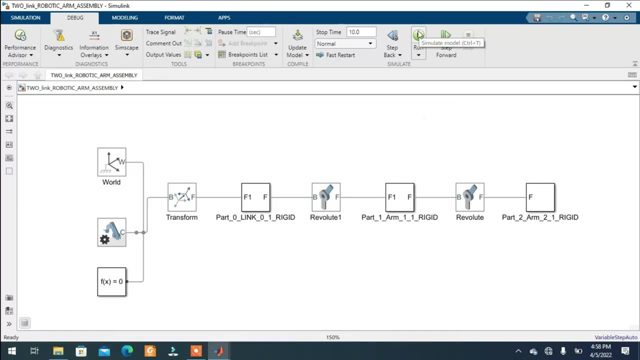 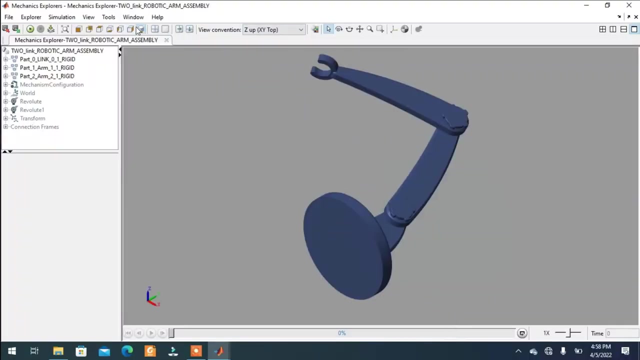 it will save as a simulink. okay, we can proceed first. let's run the model if it works or not. as you see, it is compiling now it shows us good result. here is our model in sim Explorer, in mechanics Explorer. still it is not loaded. as you see, now the robot is going like crazy wait. so we have to control this. 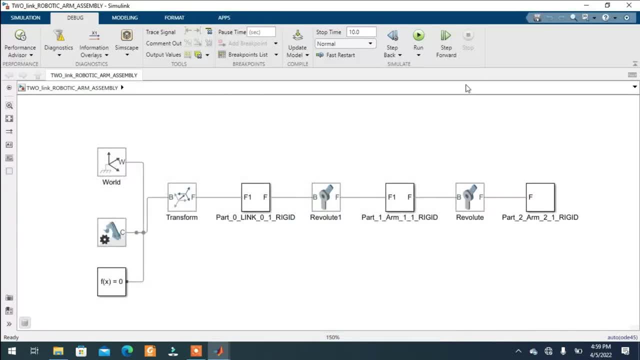 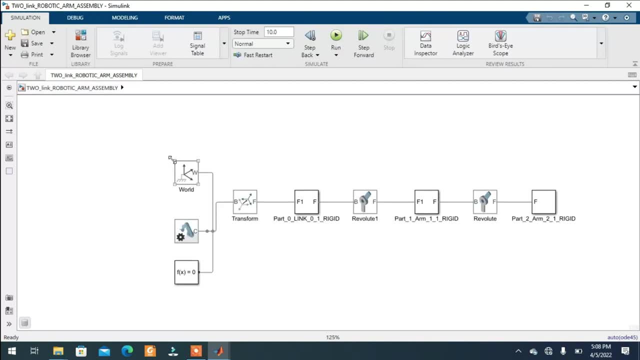 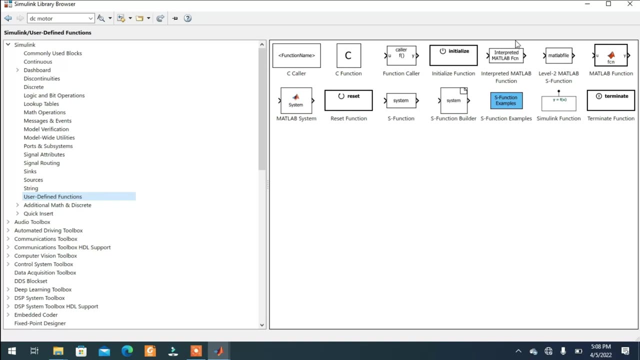 using a PID or another mechanism which we enter here now. so we have to check our results menu and now it goes back to the screen. we have some shapes already and we're on system of code error and let's add some keys into the attempt. so now we do that without 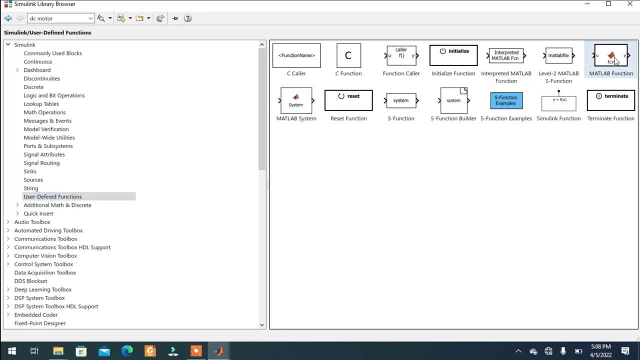 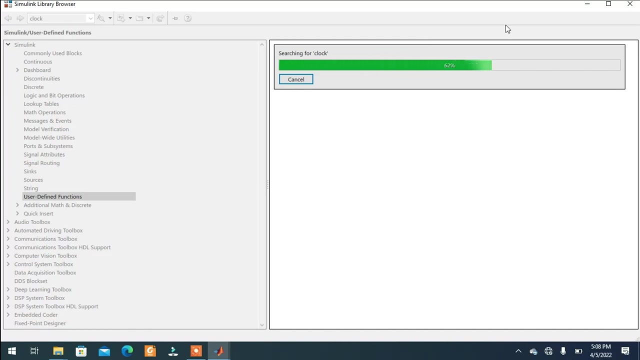 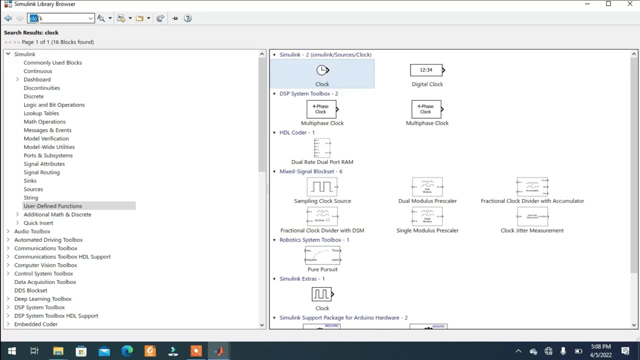 changing anything. we have to rainbow ord. but the setting is very, very simple. simply add so it at the bottom of the view with a cheat. later in it. there's a symbol, there is a button- this is the name appears on the $$ process and and right click and add to model and the other one is the XY graph. the XY graph. 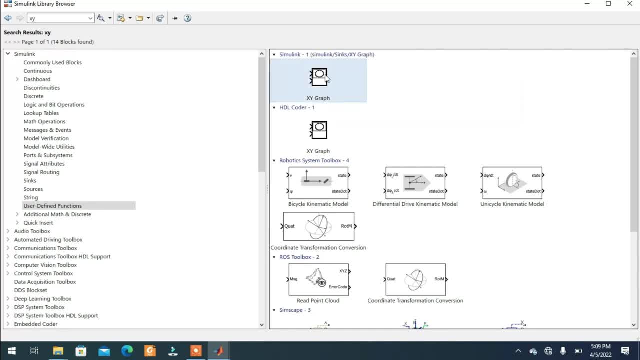 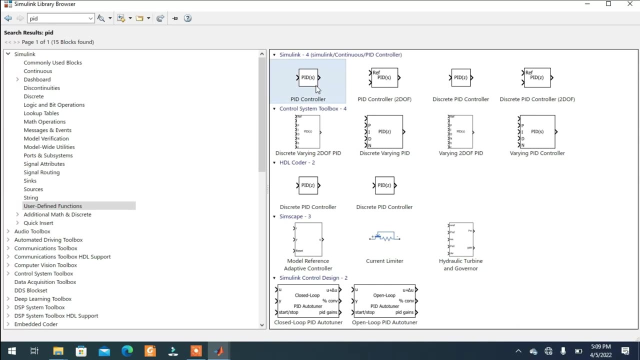 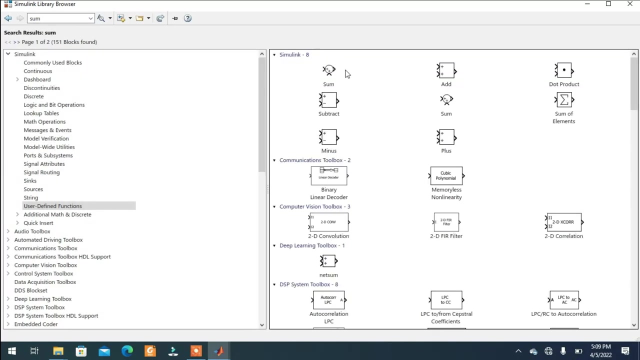 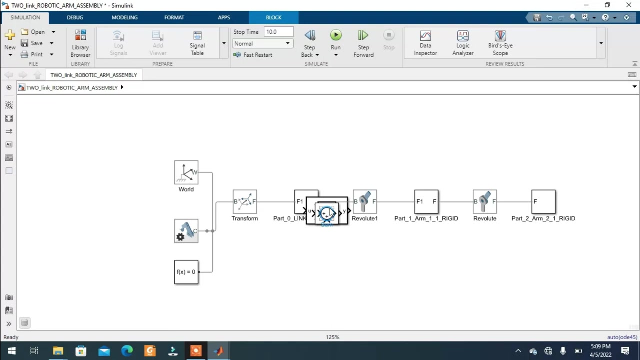 similarly, right click and add to the model and the next one is a PID controller. just type PID and enter, then the PID controller is here, then it added to the block, then the sum to subtract the error. okay, I'll position those far away from the model to do to better visualize it. 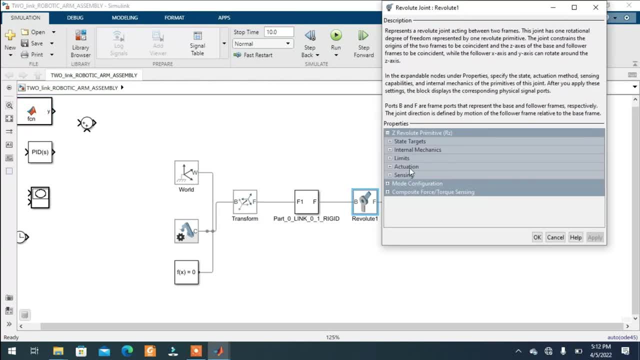 ok, this revolve joint are the robot joints. okay, this revolve joint are the robot joints. that is to be provided by inputs. the actuation and the torque is automatically computed and we have to sense the position of the robots. so, the position on the sensing block, the position 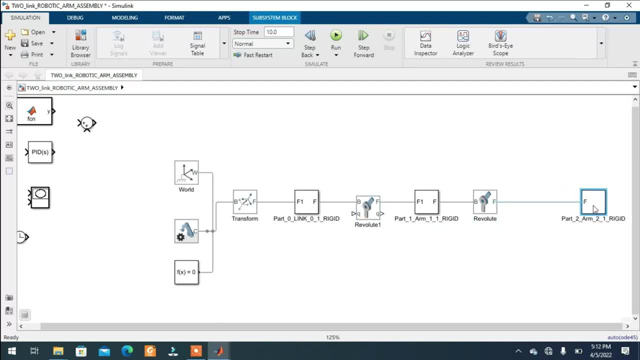 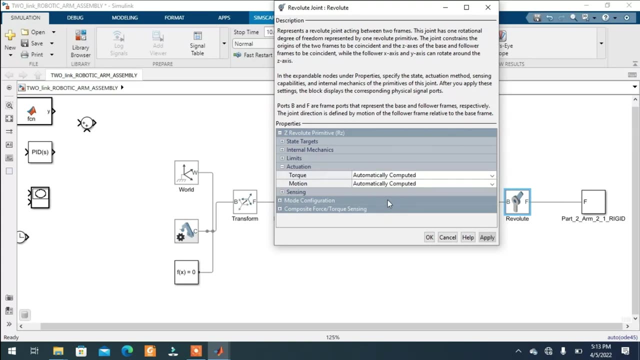 is made as an output and similarly for the second joint. for the second joint, double click on it and on the accretion, the talk will be automatically completed in the motion will be provided by inputs and the sensing, because we only sense the position of the indicator. 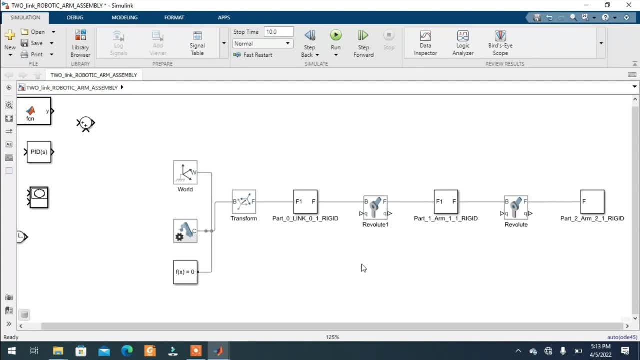 okay, double click on the basees, the empty space and typename seem to seem, skip to. então só tem que Silk Sky上 em três alças. para colocar a divisor em um filme de truque, vou fazer um vídeo de crew iniciado num Artem, Westburĩ. 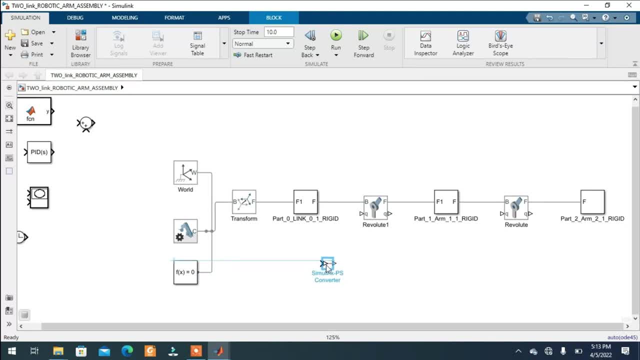 okay, double click on the- this is the empty space- and type simp through. seems. keep to sim. skipper 2: dance in every employed withöhne. apressa ut device na presa, na opção, até clique um muffin, no royalties. Simulink to physical converter and physical to Simulink converter then. 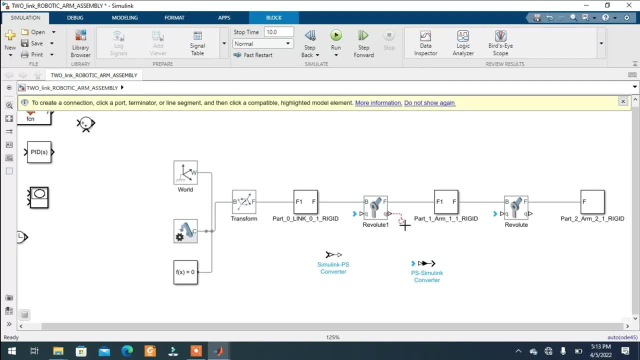 connect this output to this and connect this. similarly, copy those two files and the memory name, the joint, the first joint one, and join to copies these two and connect them. and on the empty space type in this will be as an input and outputs connected the outputs copy and paste. 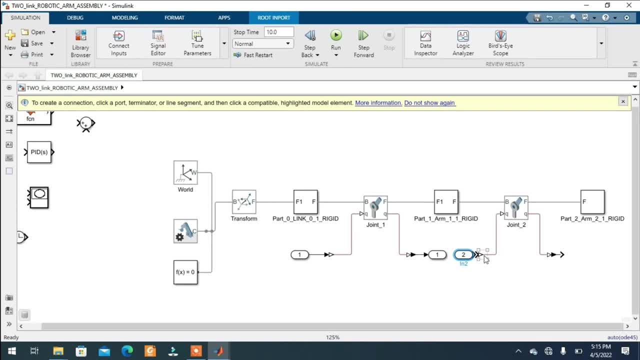 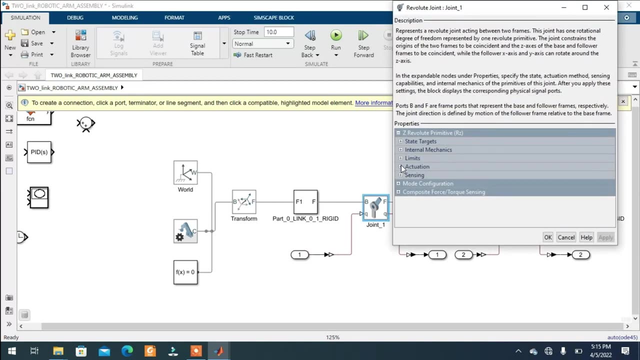 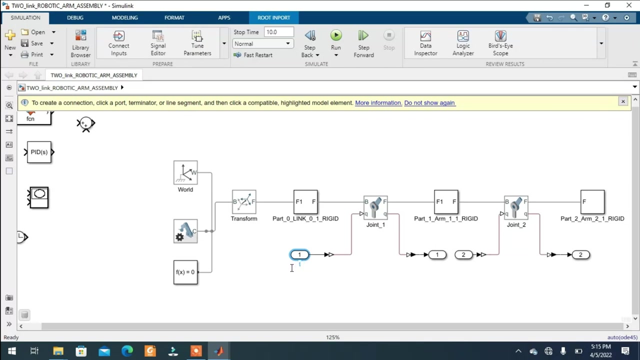 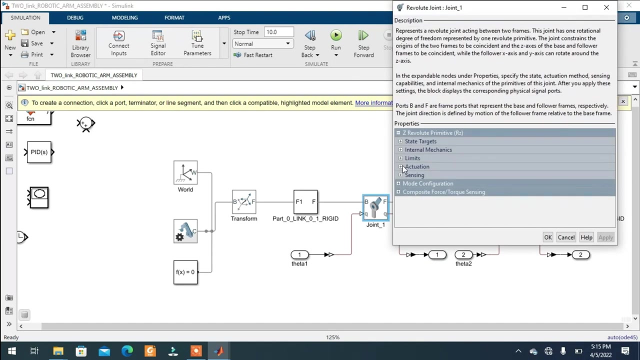 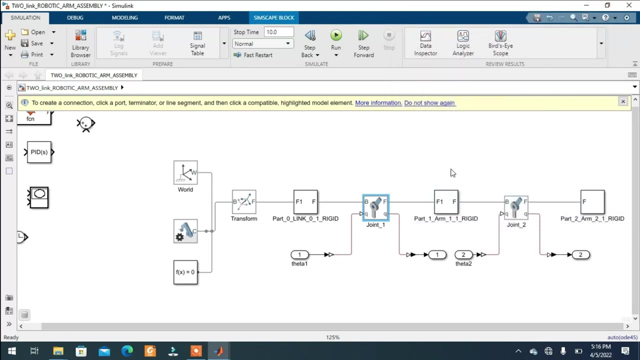 connect this two. make sure the position is only the sensing, is the position only and rename this as theta one. and for the second input is De cutting and outputs when News first output us fitted, the other one and this type poverty one end inputs Annie, is the output, is the outputs. name z first output, us, the third one and this yield one and the output. therefore reckon the output was called Pgun, the output of the Pgun, the output first output and the output i. we name the first, exactly, force between MZ. we name the first output is theta desired 1 and the output. i will name the output z, the output as the third. i will name the only individuals. again, same standard, input one, fifth one and this output is bugger homer, same standard and the outputs j2j, two will be working on the remet, the output fmром, the components. évidemment, it's going to interrelate thick기를In this strip which will represent as output Macro. this is the memory, my link, the 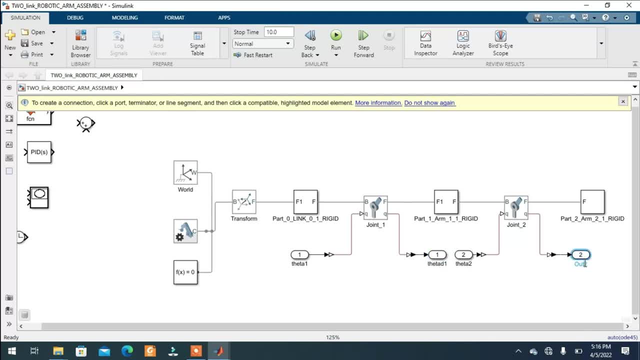 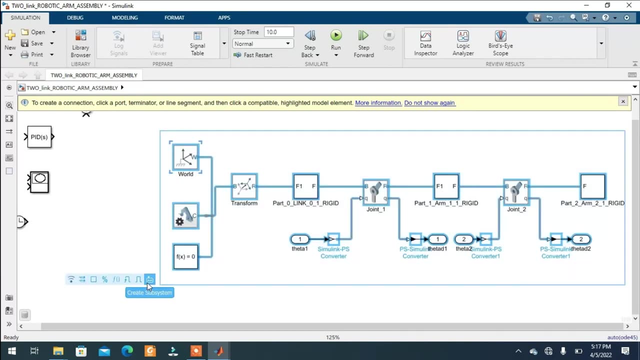 pending inputs is the memory of acrylation, of memory, like i, altsanus, j0. what language this is 노, the network f, And this is the desired tool, And select all these and make it create a subsystem, Then rearrange this. 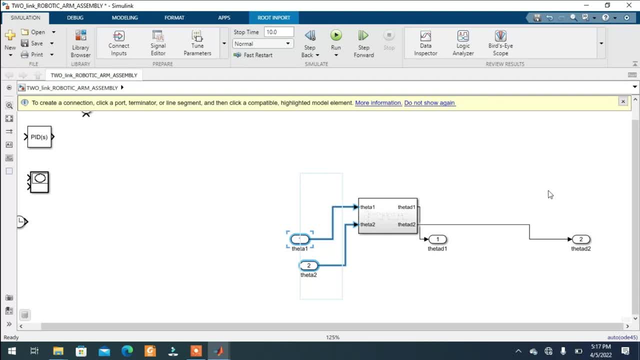 We don't need those, So we delete these outputs and inputs. Then we need only the subsystem that holds the robot mechanical model. OK, Then we will go to the others. First, save the file, Bring the function block And copy and paste it three times. 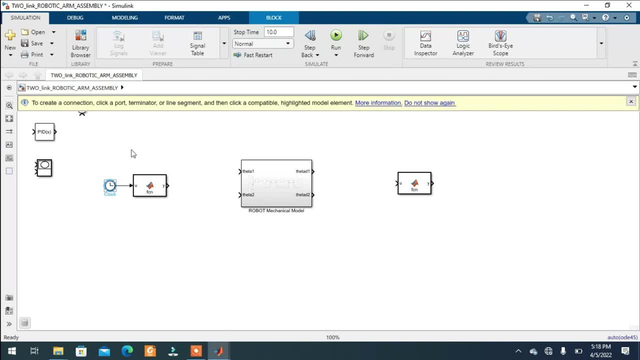 Then connect the clock. Arrange the same PID to better location for connecting the lines. We need two sum Two, one for theta one And theta two. Then we need two PID controller. Arrange it properly, Then Then double click on it. 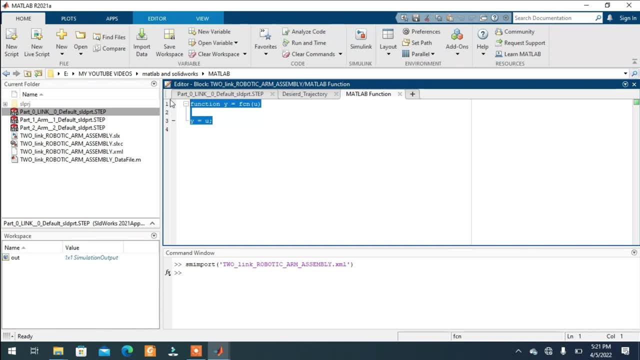 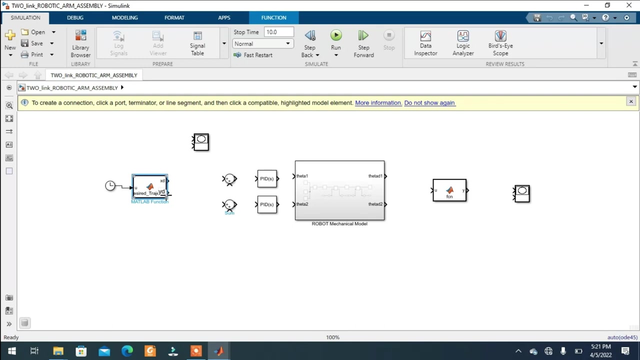 Double click on the function. Double click on the function and write this code. as you see, This is the desired trajectory And with the input U, After we save it, The block will be changed into two outputs, With one output And with the other one. 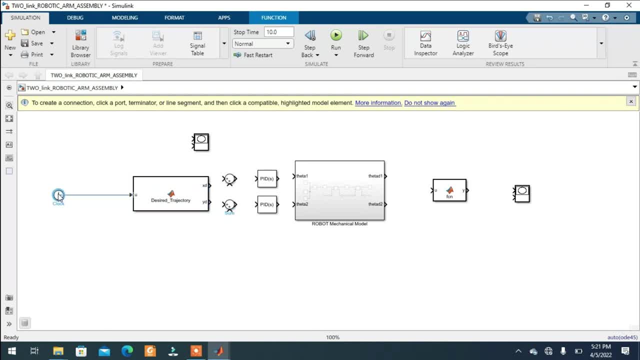 After we save it, The block will be changed into two outputs, With one output And with the other. The two outputs are Xd and Yd, And also we name it as a desired trajectory. As you see, These two outputs are connected. 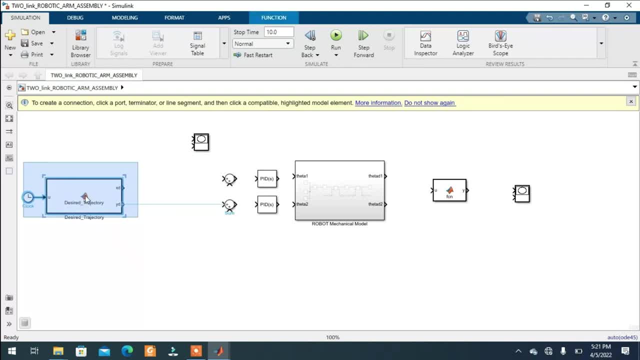 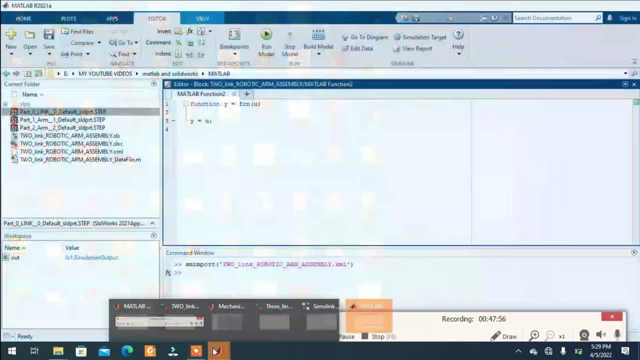 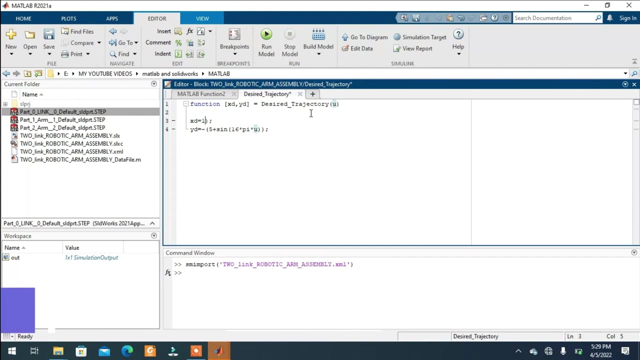 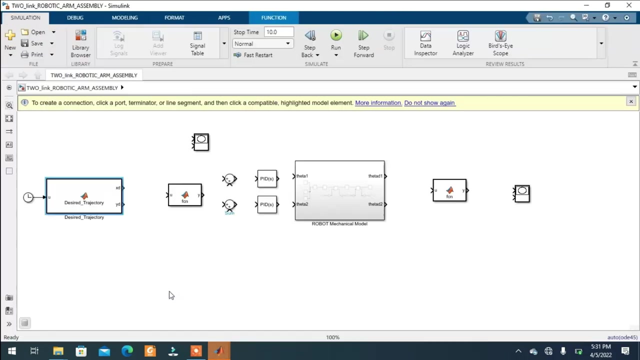 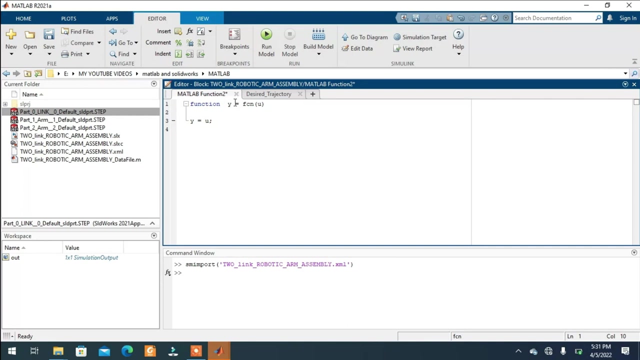 With the same block, Then connect the clock. Thank you. Thank you. Then double click on the function tool and rename this function name. First, the outputs are theta1 and theta2. with the name of the function is inverse kinematics with an input xd and yd. 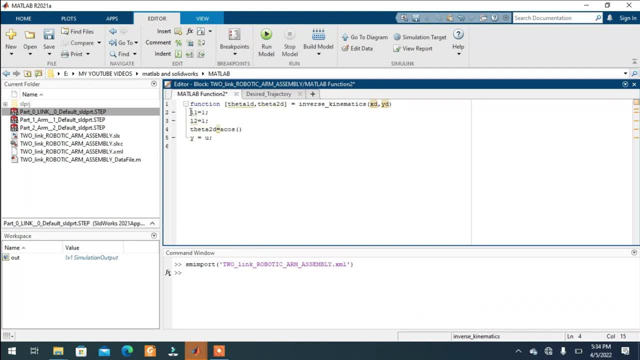 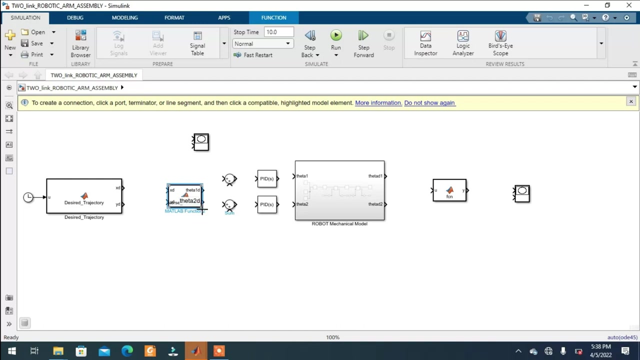 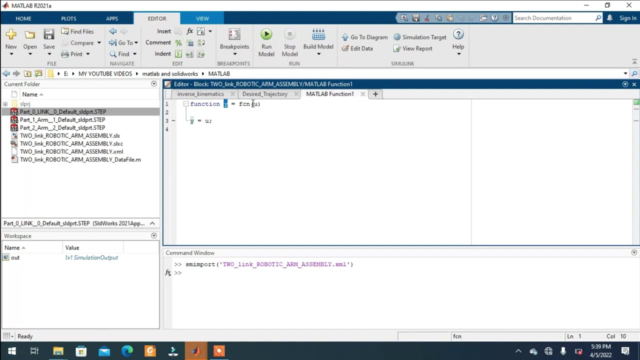 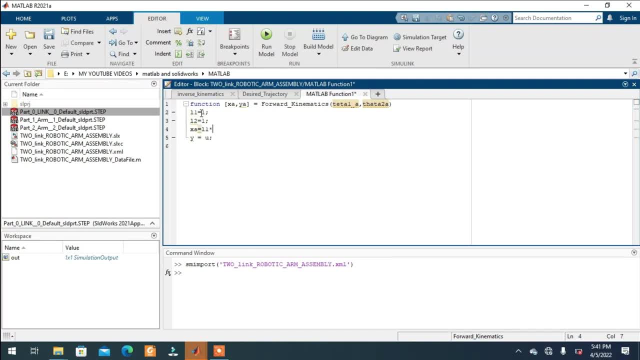 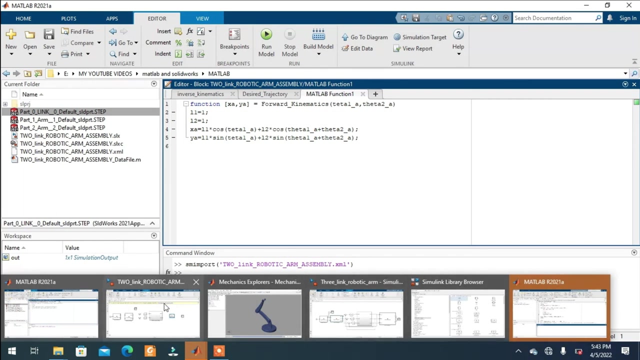 Then give the length and write the formula for the forward kinematics. Then give the length and write the formula for the forward kinematics. Then give the length and write the formula for the forward kinematics. Then go to the simulink module and rename it as forward kinematics. 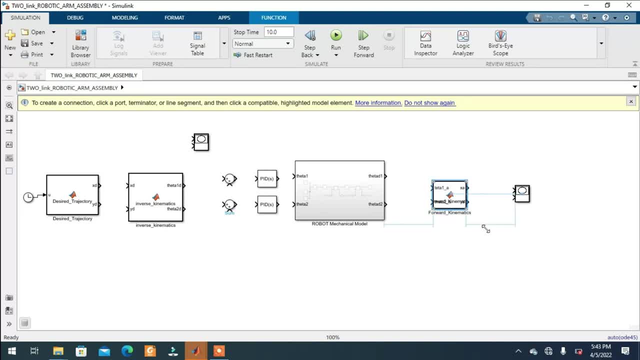 Expand the block, And now we are going to connect every element. Then xa, connect it with xy, Then this theta desired is connected to the forward kinematics block, Then the PID controllers will be connected. First, connect the xd and yd. 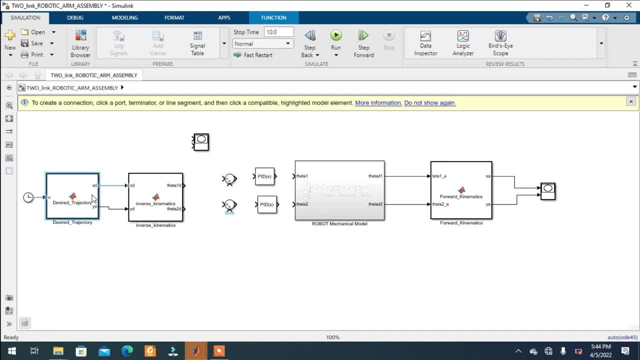 Resize it, Then the PID controller will be connected. Connect these two. Then connect the sonar block- Here we have the same procedure, Then the workpiece at the front, And here we have the block at the back. Also connect these two. 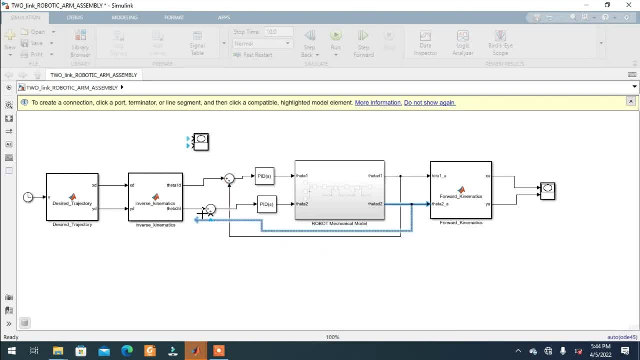 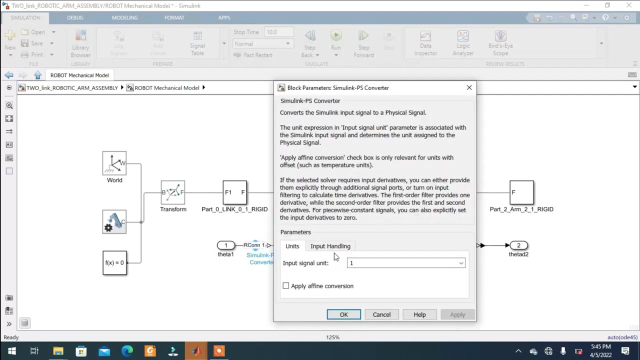 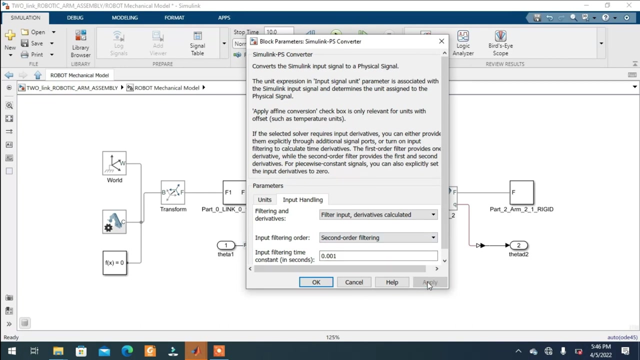 Then drag this, right click and drag this and connect to the same block And connect this xy graph. The xd and yd are the desired trajectory. Then from the desired trajectory, using xy plot, we can see how the robot will go And make sure, on the mechanical model, connect at the input terminal, the ps converter. 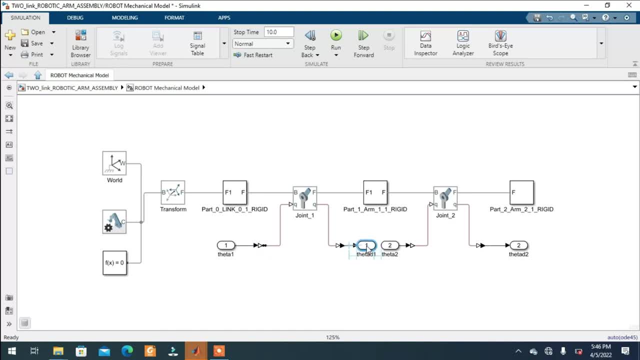 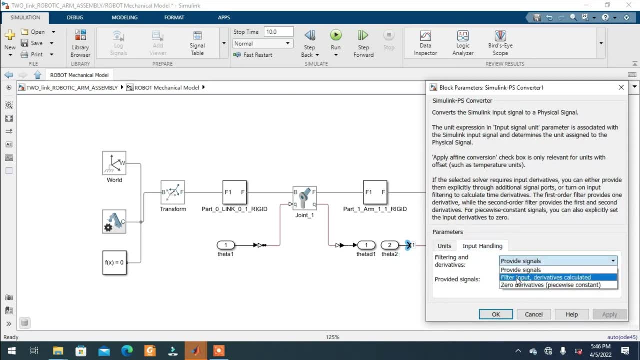 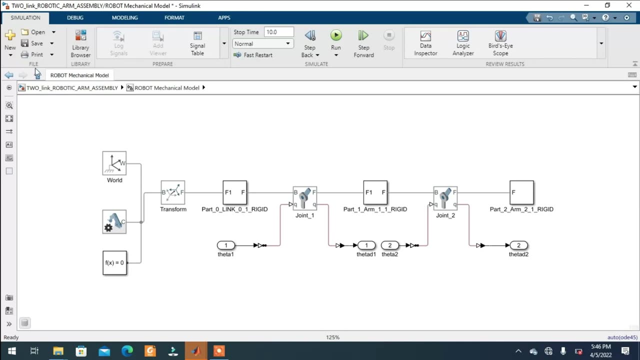 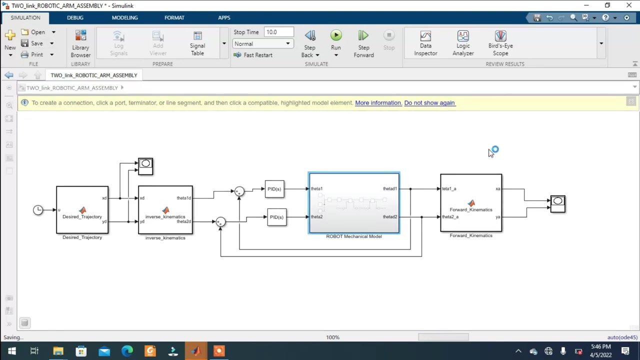 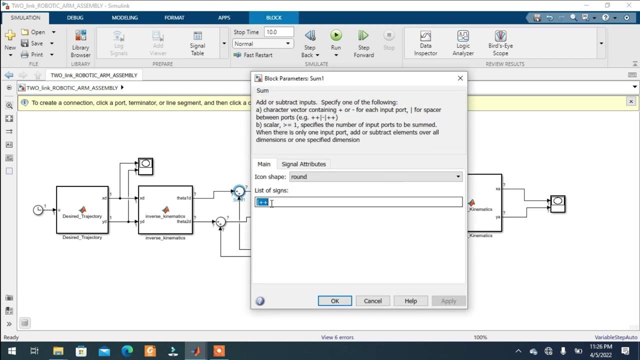 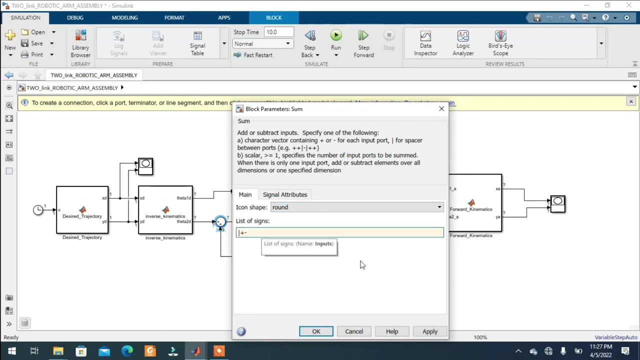 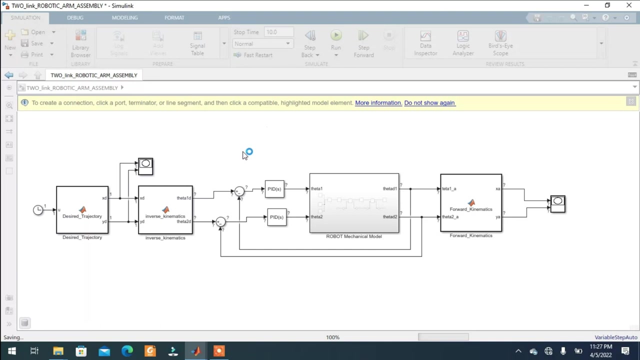 Make sure the second order filtering is correct And make sure the filter type is on Unless, otherwise it doesn't work Since we use ode 45.. Make sure the filter type as second order filtering And click ok. As you see, we have to rename this as minus, since we need the error. 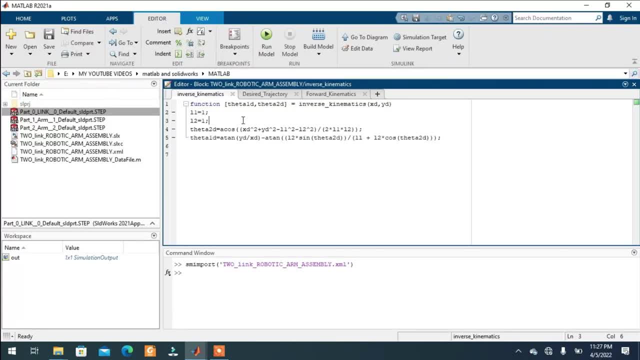 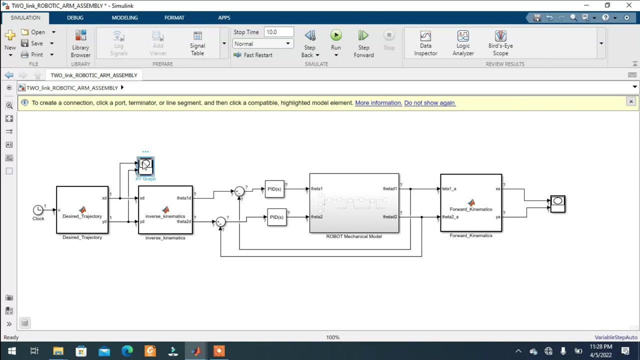 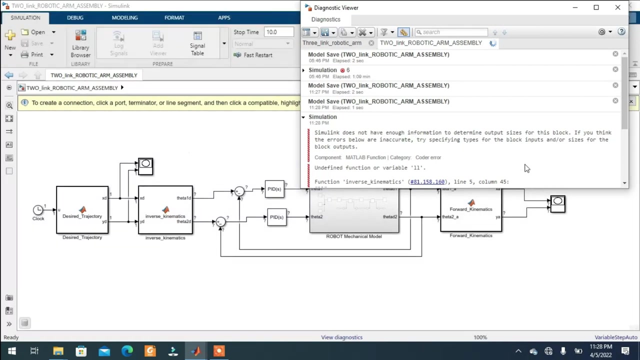 Then save it. Ok, Now we can see that our code is correct. Make sure our code is right And we didn't make any mistake. Run it. It's now compiling. Ok, there is an error, As you see. Ok. 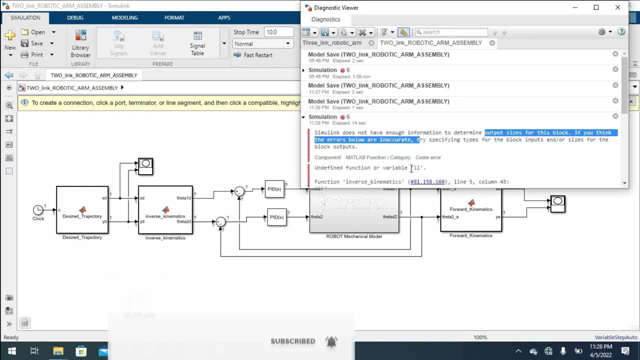 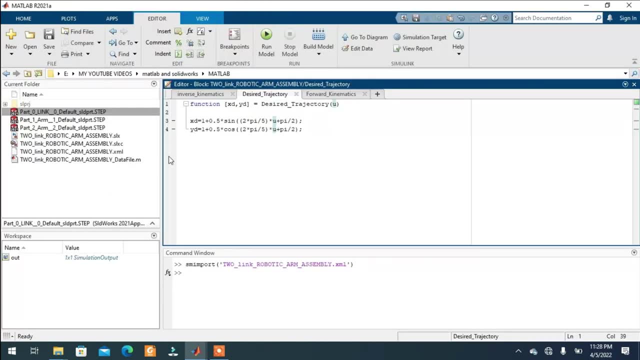 There is an error on the code, The undefined l1.. So we go to the inverse kinematics, Then the inverse kinematics, Under the inverse kinematics. There is some error. Ok, Now we can see the error, Ok, Ok. 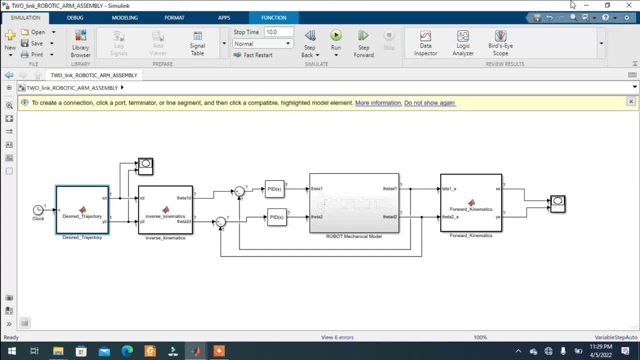 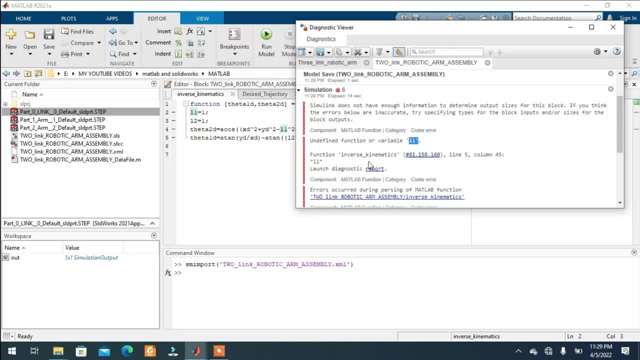 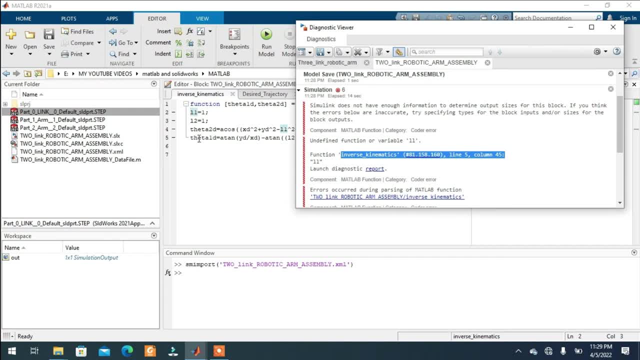 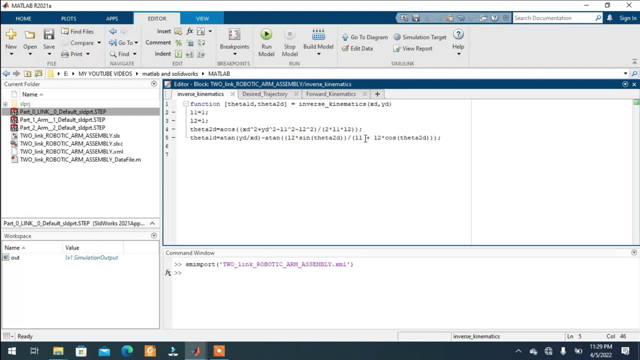 So it guides us to this position On line 5, and column 45 is around here. Ok, Ok, Ok, Ok, Ok here. as you see, when we select it, other L1 is not highlighted. when you select this, they all are highlighted, but not this one, so make sure, rename it, then save. 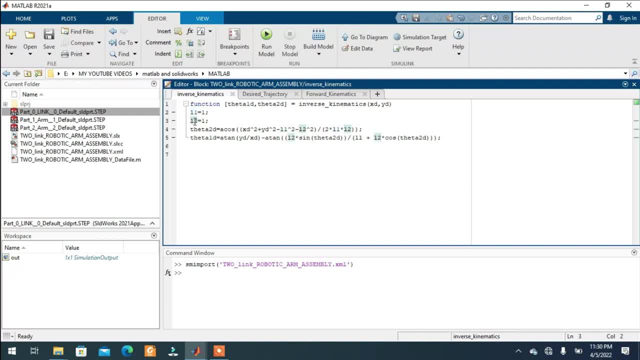 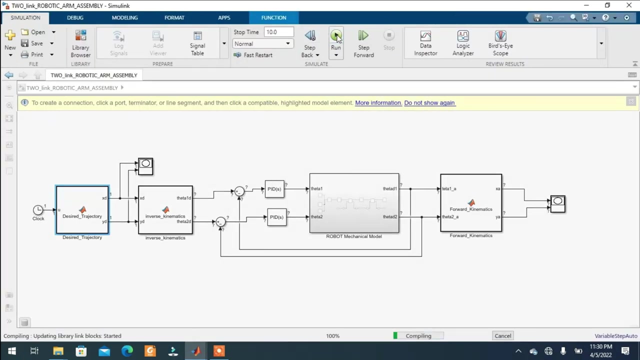 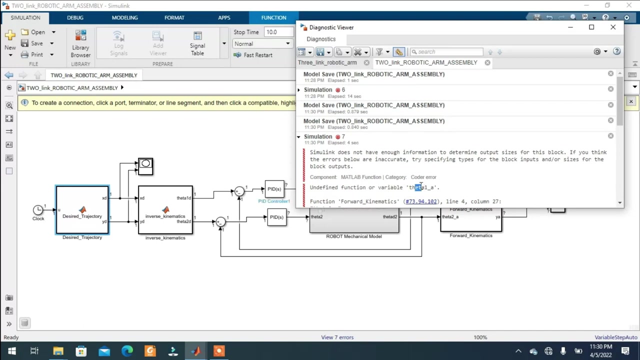 it now to check it: click on the L1 and still doesn't show that on the line 5 alone is not highlighted. so copy it and paste. one and L are nearly similar. that's why I'm confused here. and let's run the model still, there is another error. okay, on the forward. 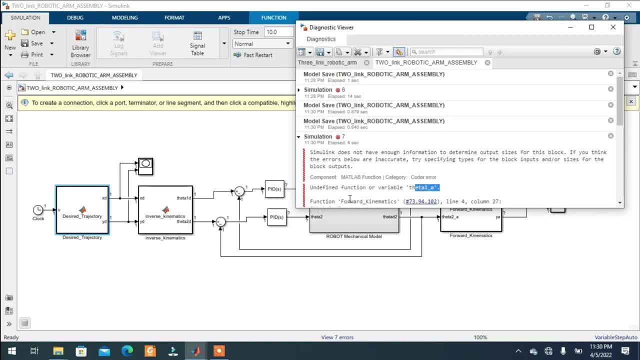 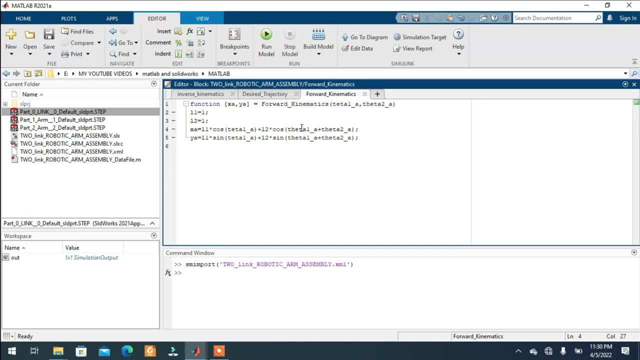 kinematics, block theta1a. the variable theta1a is not defined. on the forward kinematics, the fourth line, theta1a. as you see there is a an error here here. then delete this H. now it seems good here. there is another mistake. now it's. 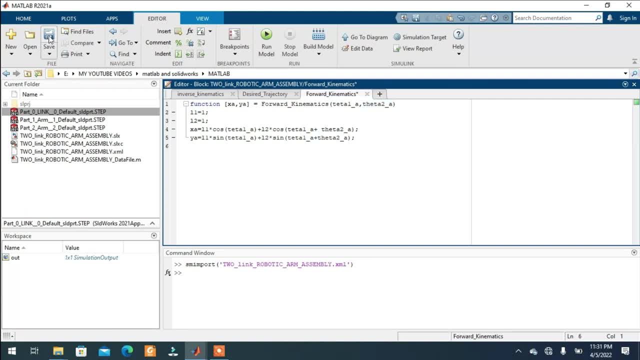 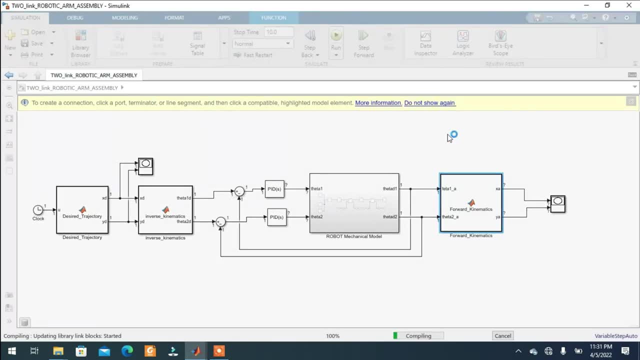 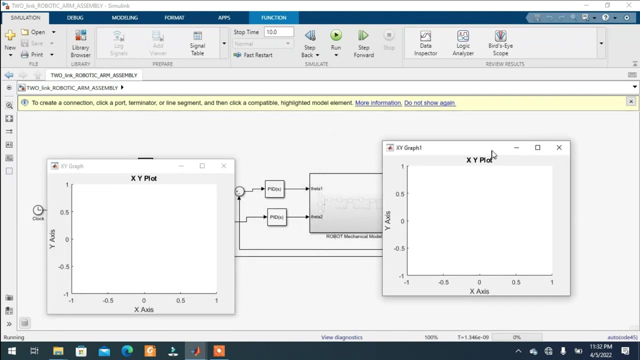 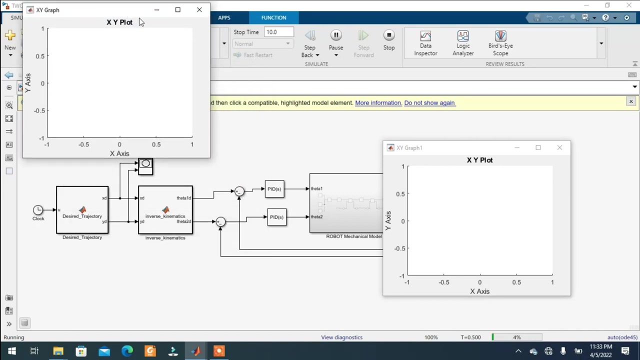 better. okay, save it and go to this and run. as you see, the model is working properly, the time is working, and now we are going to run the model and let's see how the time is working. and let's see how the time is now running. the model is running, but it is so slow. 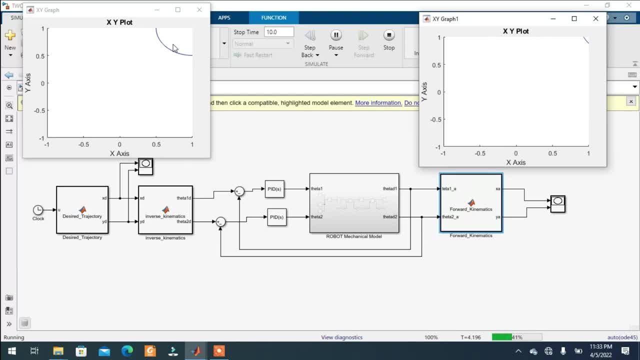 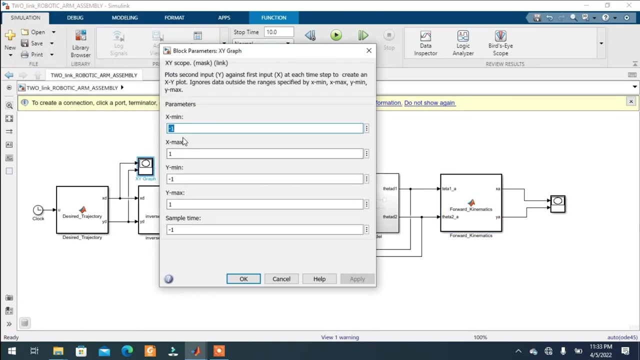 and, as you see, the input, the desired input on the xy graph is shown. the output is also shown. but it is cropped. so we have to resize the xy plot, since the xy plot is only showing us from positive one to negative one on the both x and y axis. so we resize it as that by first double click. 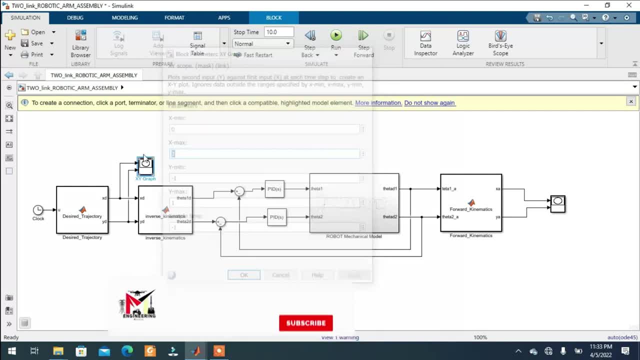 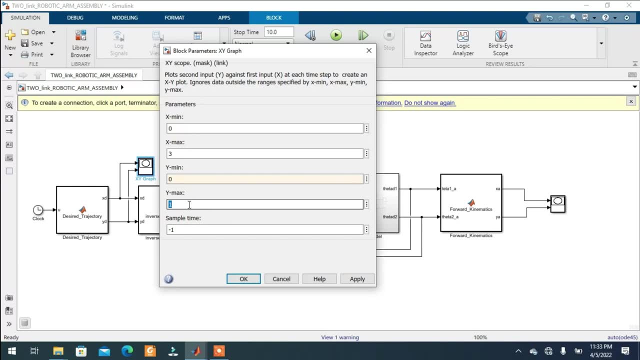 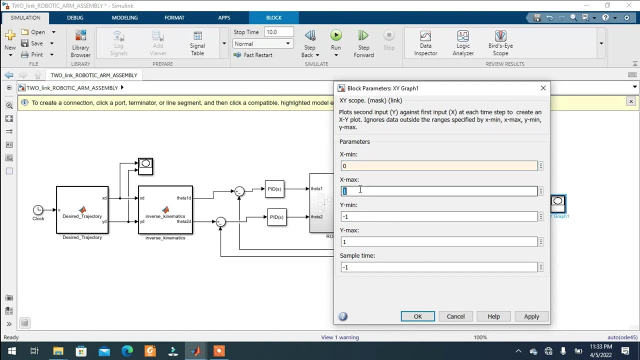 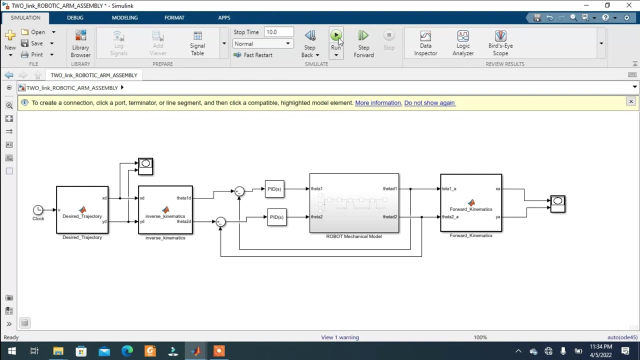 on the block and the minimum will be zero and set the maximum to three. and again for the negative side, set it to zero and one. and for the output, similarly, as from this diagram, you see sample time as minus one that will be inherit the previous sample time from the model, not the actual negative one sample time. 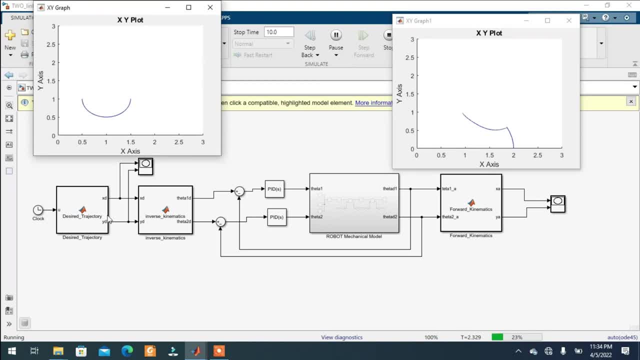 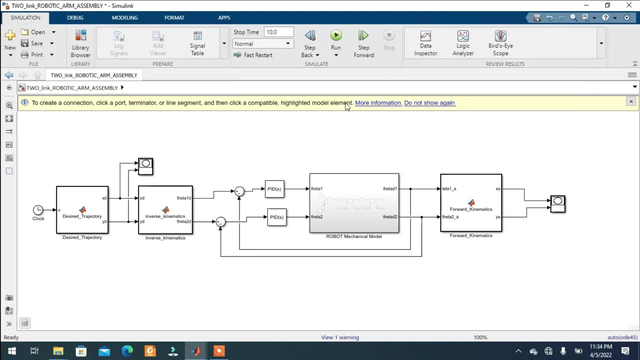 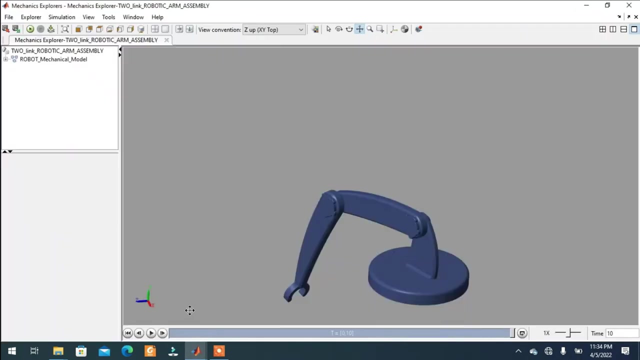 as you see, the output is nearly tracing the input trajectory, but there is a. clearly there is an error. so we have to turn this pid controller to better mimic the desired trajectory. okay, to turn this pid, double click on the first pid block. as you see from this, a mechanics explorer, there is a smooth animation, but this simulation is not correct. so 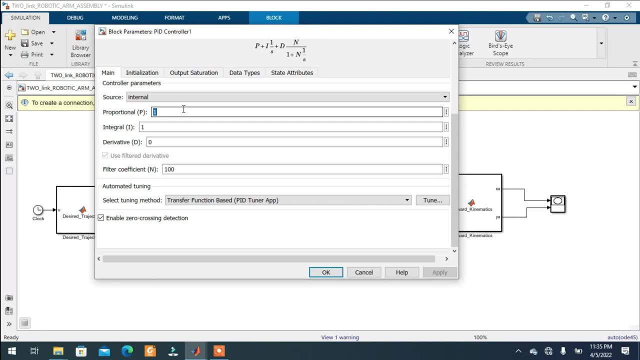 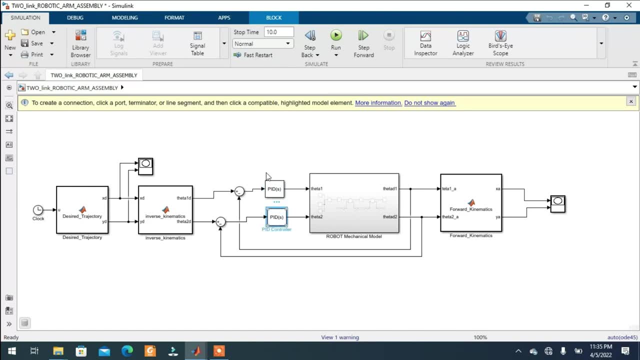 we, with this pid controller, block parameters. we have to change some components or samples and some some parameters to better see the outputs. so that makes the proportional as 10, the proportional gain as 10 and let's see how the proportional change, the proportional gain, will change the response of the system. 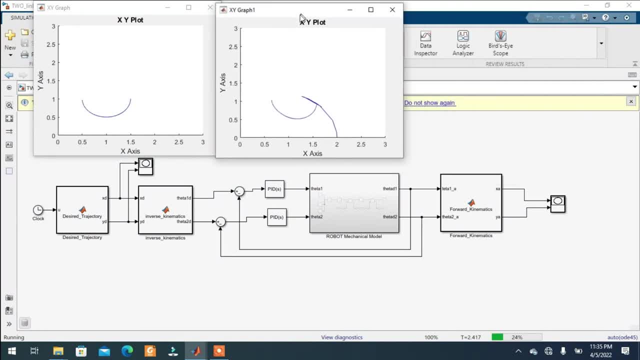 as you see from the plots. here are the two plots. if you compare it now, we get a better value from the previous one. the proportional gain will reduce the steady state error. the proportional gain will reduce the steady state error. if you compare it with the previous outputs, the steady state error is very large. by just tuning. 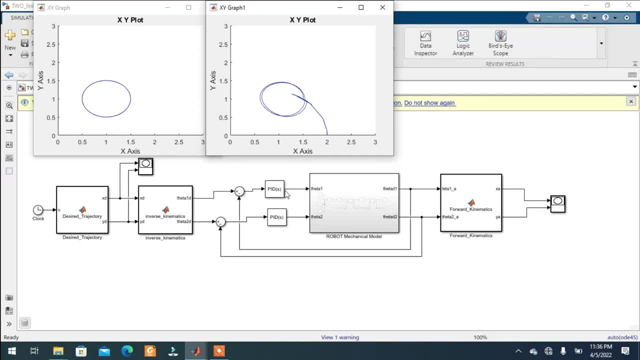 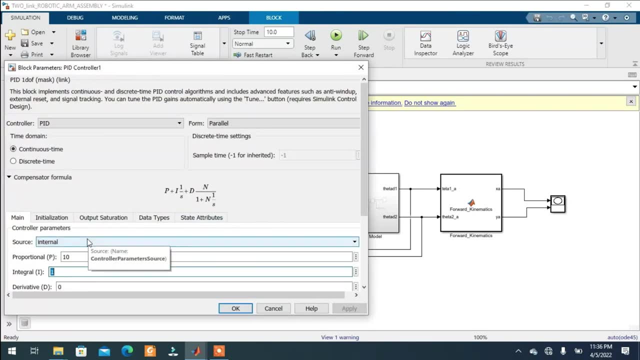 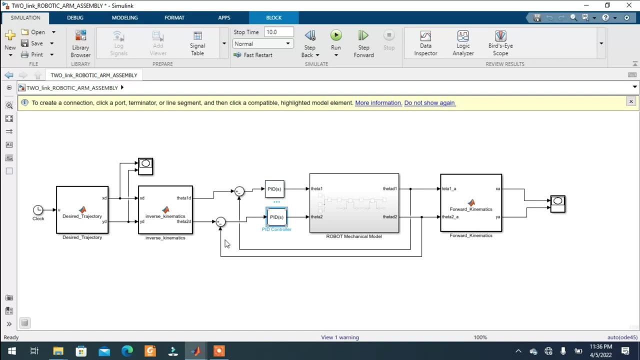 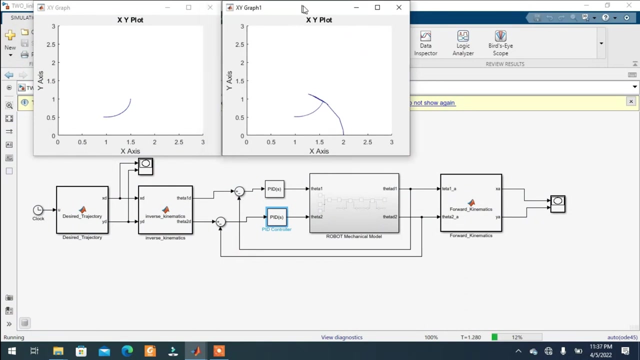 the pid block parameters on the p: the pid block parameters, the p only. of the pid block parameters, the p only. we can get better. so again by changing another parameters, like the integral parameter to 20, we can get a different results. okay, let's run it and see how it will work. 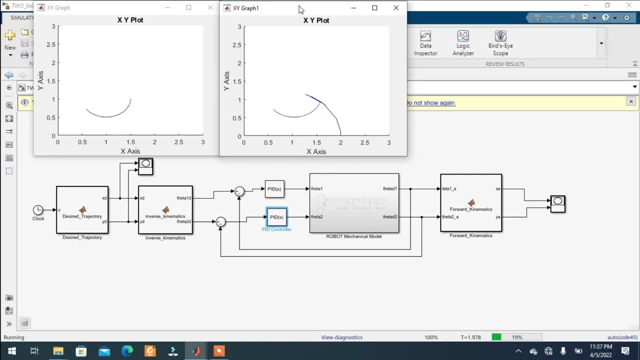 as you see from the input output plot, this simulation takes a little bit time. okay, now the result is better from the previous one. the error is now eliminated. there is no overlap between the lines. okay, now, let's go to the next step. okay, let's go to the next step. 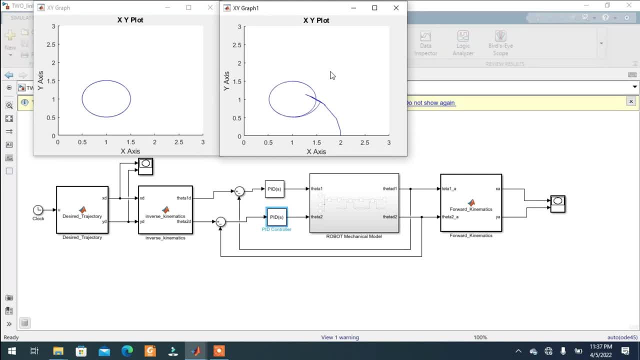 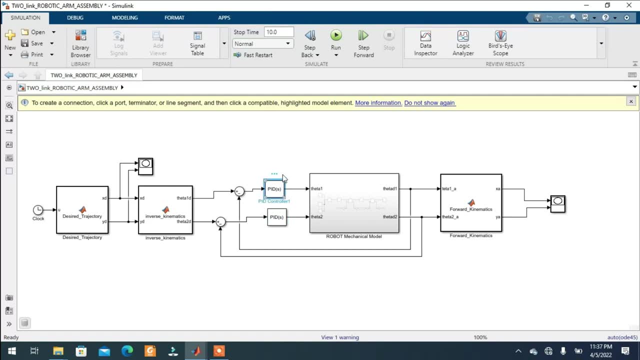 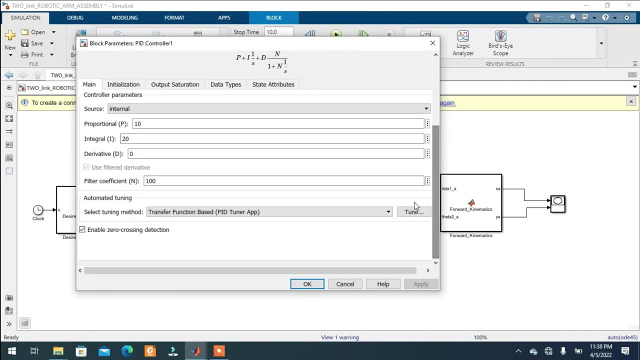 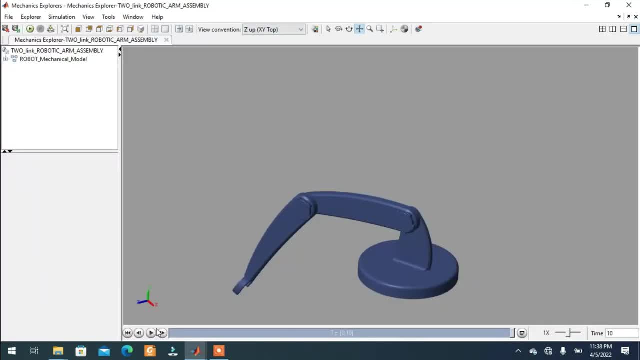 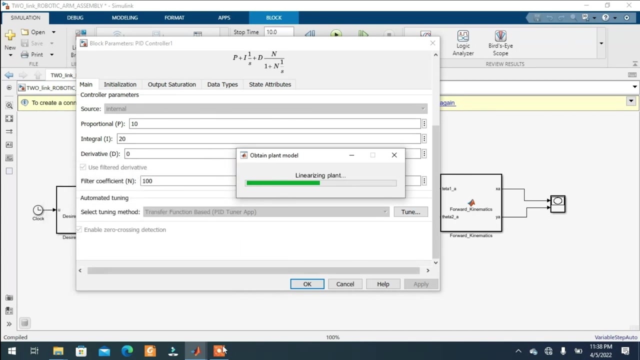 over the robots. okay, when we press the two button there is a mechanical robot. mechanical model is nonlinear model, so PID is linear model. so we have to change this nonlinear model into linear, so PID, the PID block by itself will linearize model and approximate it to a linear one. 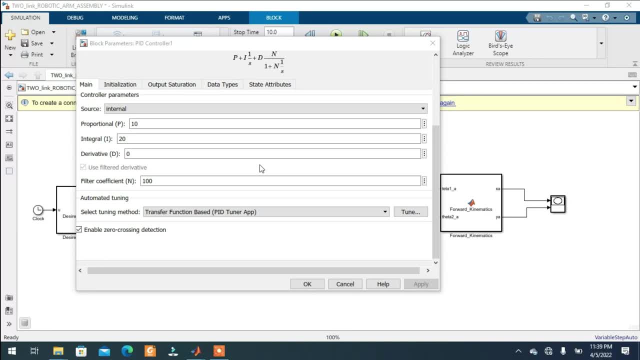 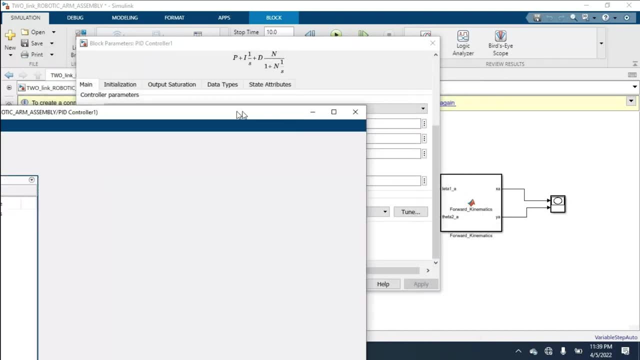 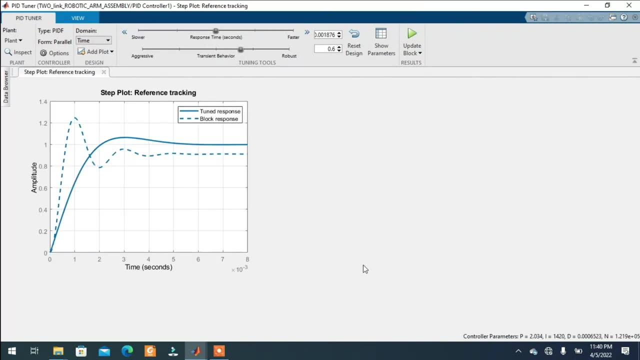 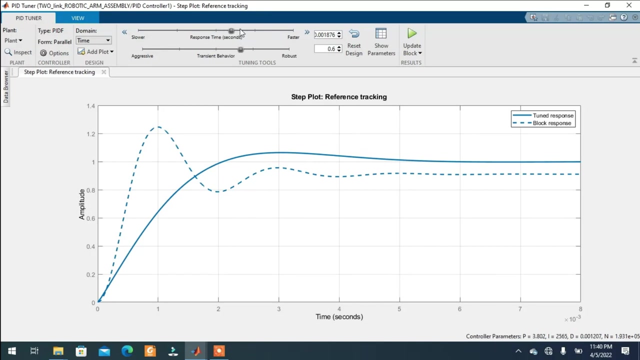 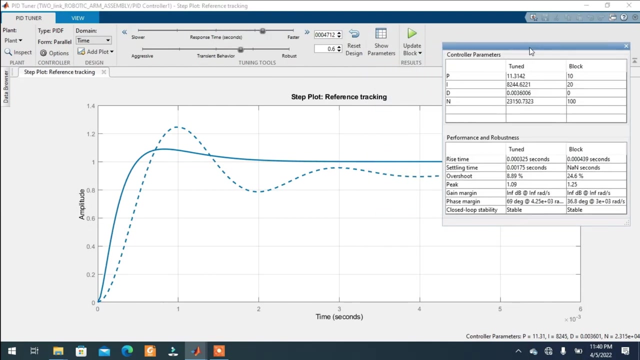 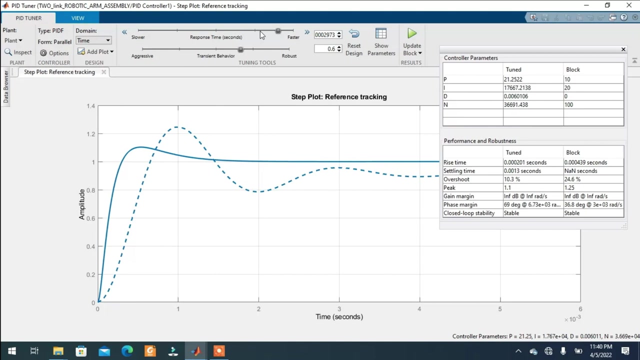 okay, take some time. okay, now the tuner app is opened, the PID tuner app. as we see the previous block response and the tuned response, we can change the response time faster or slow, and We can also play on the behavior of the transient response by just sliding the sliders at the top. 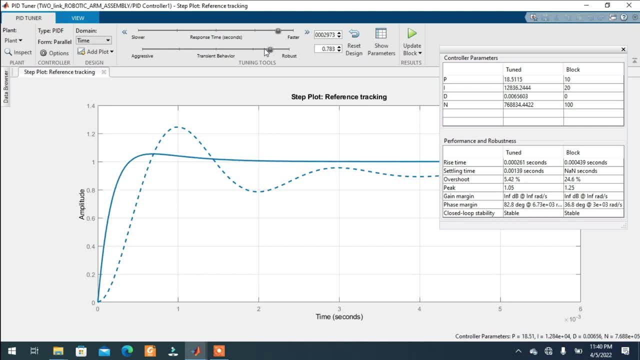 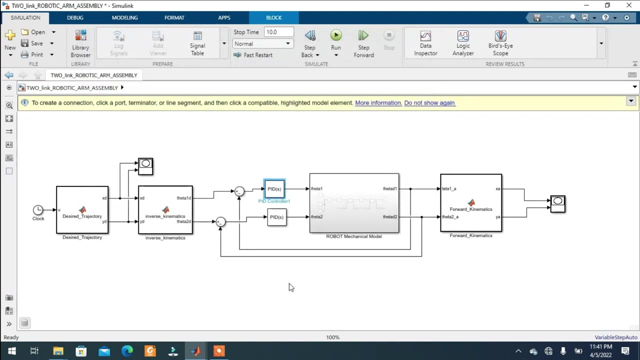 And you can see the overshoot, settling and rise time on the show parameters. Then, if you get a better control or a better results, you can update the block just by pressing the update block button and close this window. Then, as you see, the PID parameters are updated. 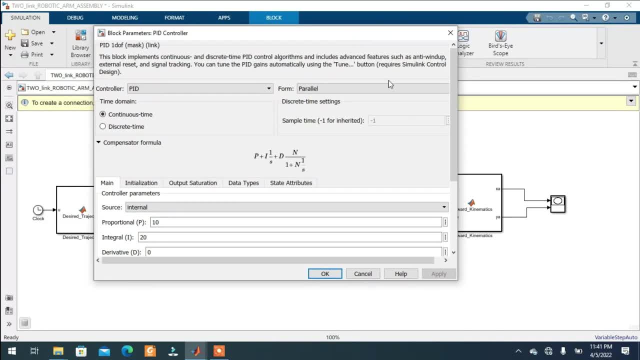 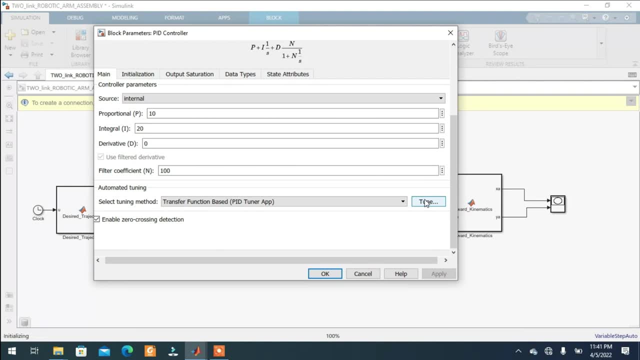 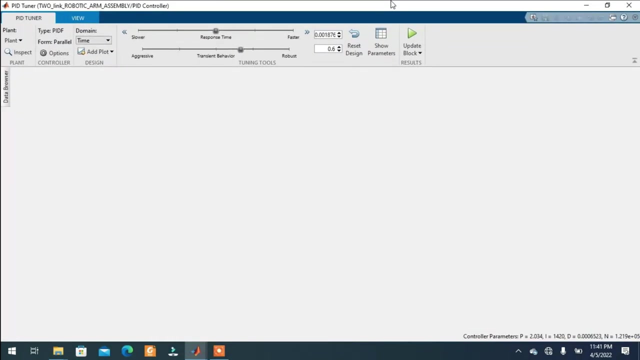 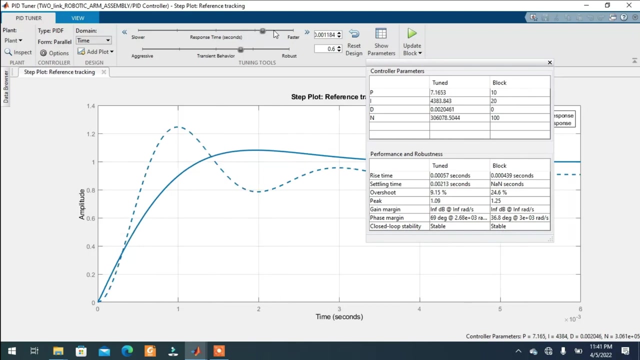 And for the second controller we will do similar procedures. Just press tune button and the plant will be linearized, And after linearizing it it will pop up the tuner app And by sliding the sliders we can get a desired reference. 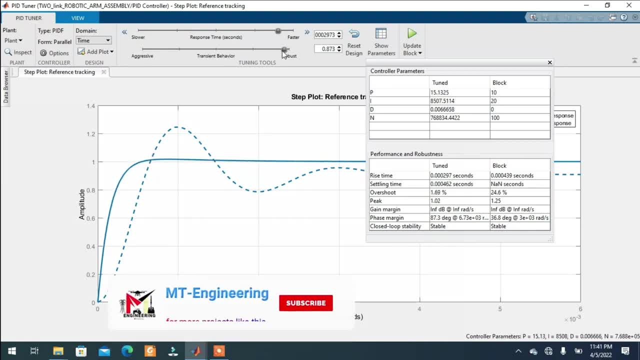 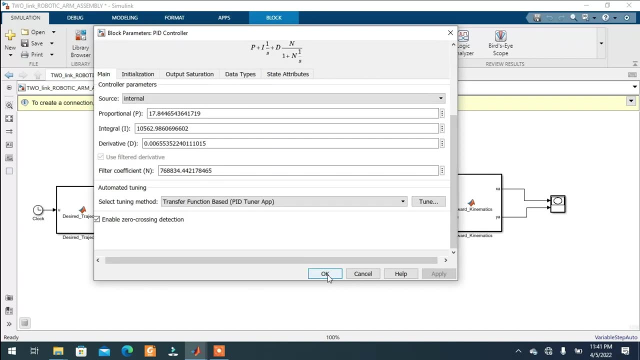 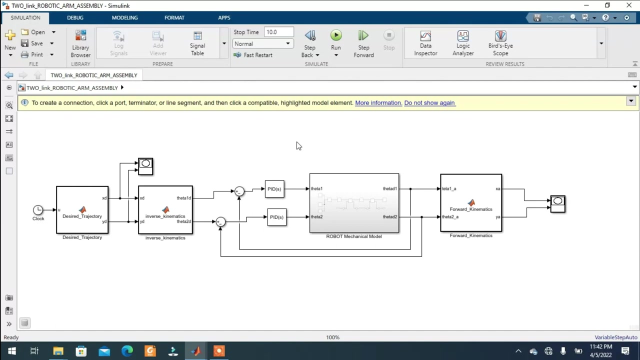 As you see, I make it faster and robust, But it is not an ultimate. There is 4.13 overshoot. That is very little. I make it just for better simulation, not the real one. Then save it And run the model. 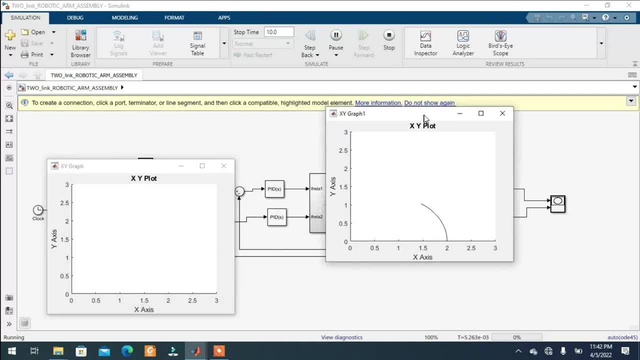 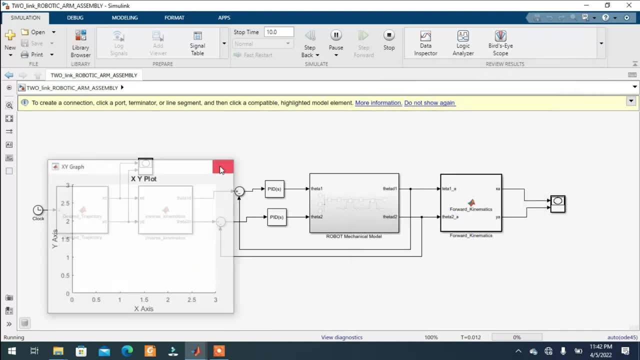 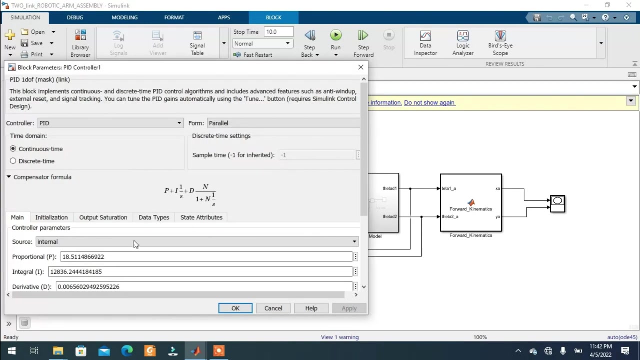 As you see, now, the time our computer, my computer, is stuck because of the D controller, The D parameter in the PID block takes much computationally intensive And we have to make it to zero, since it is very computationally intensive Even if it is very small number. 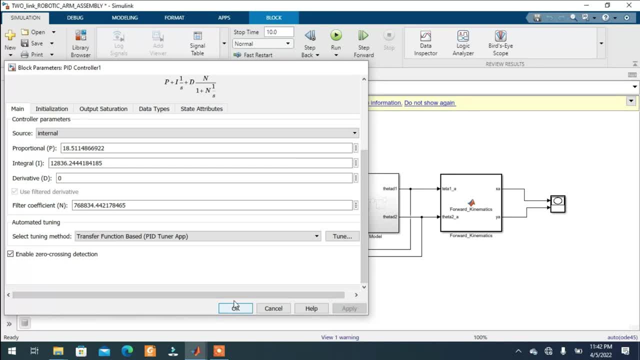 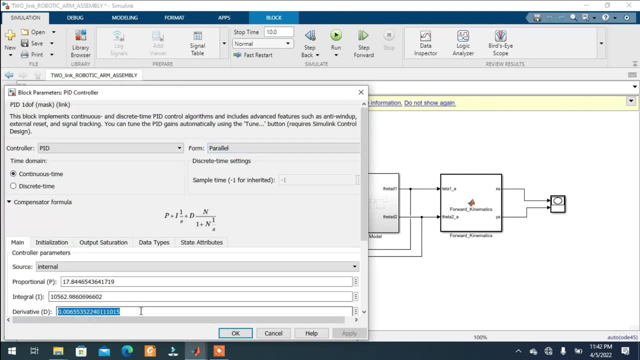 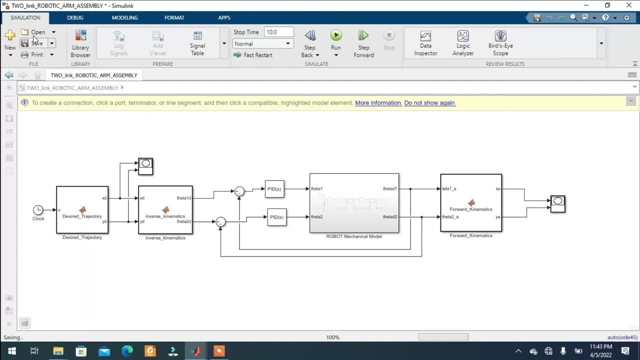 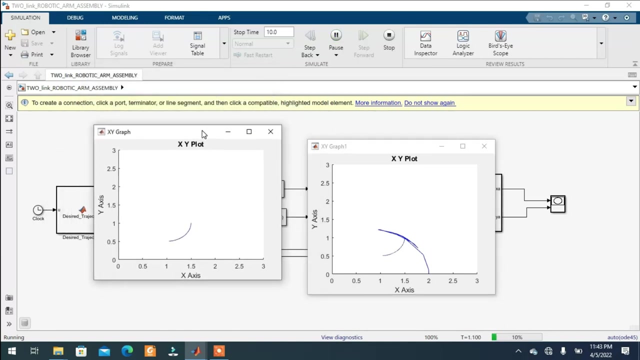 It takes much core of our PC. So make it zero Or you can use a PI controller Now, save it and run the model. Now, if you see, the model is running faster than the previous one, Since we make zero on the D parameter of the PID controller.